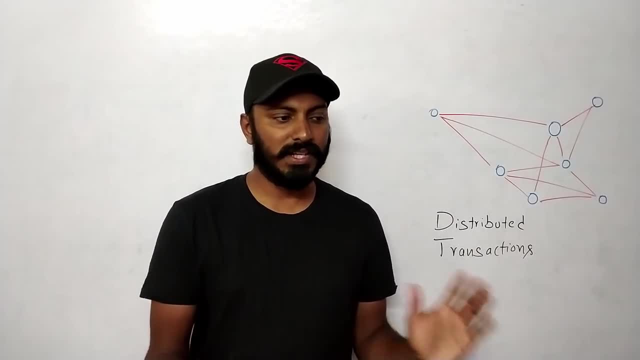 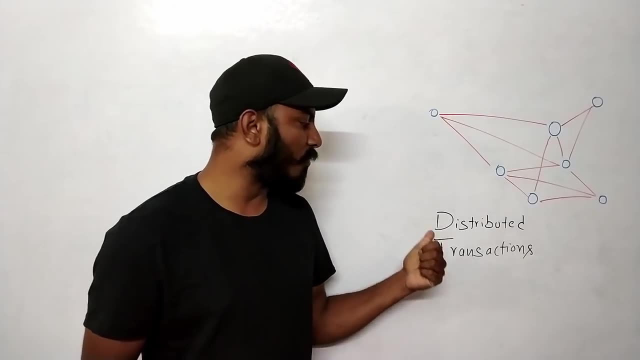 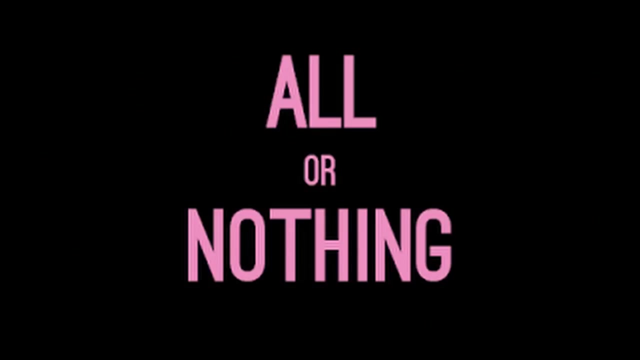 optimistic logs will actually help you to implement transactions in database and non-database kind of environment. In this specific video, we are going to talk about more about distributed transactions, Because we learned that in database the concept of transaction is all or nothing, Basically when. 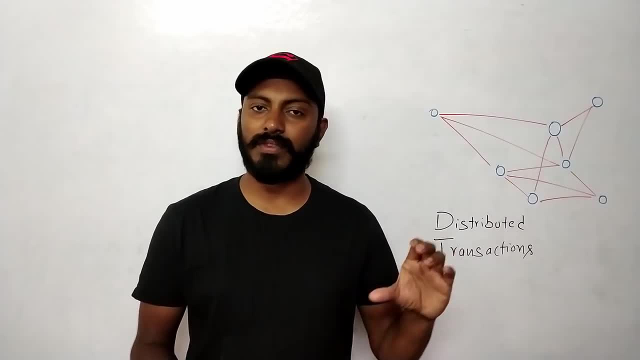 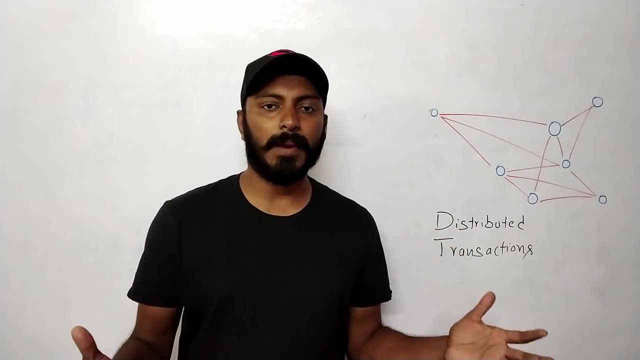 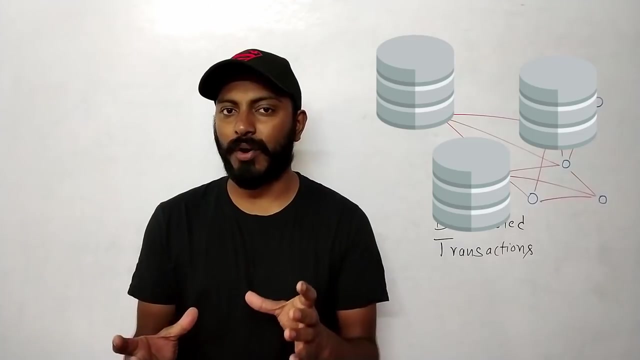 you have so many queries and updates, we treat all of them as automatic block and then we always expect all of these to pass or none of them to be executed. But think about it: if we don't have one database and we have so many queries and updates where we want to treat all of them as atomic, 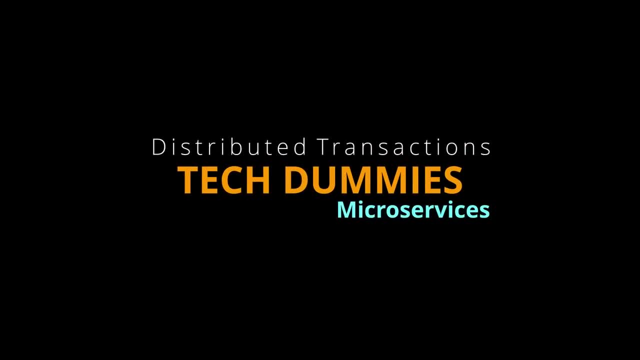 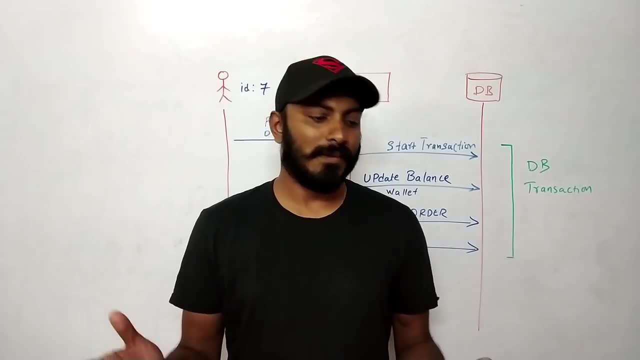 then how do we do about it? I hope you guys know different kind of software architectures. One is micro service architecture, one is service-oriented architecture and the other one is monolithic architecture. Monolithic is old and it is gone, and service-oriented architecture is being used somewhere. and the most popular one. 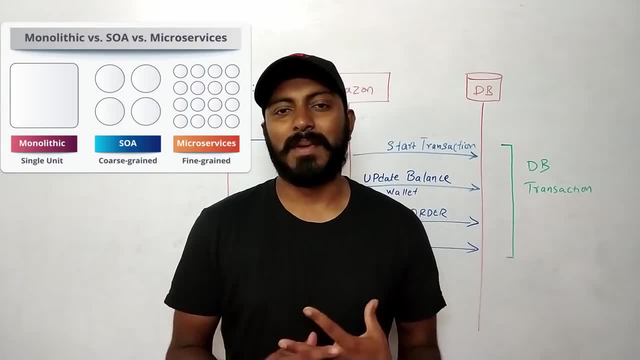 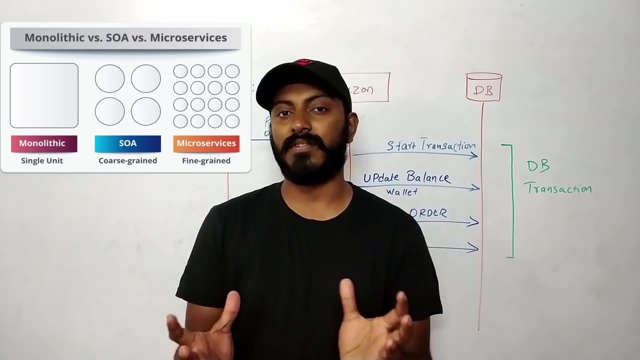 is micro service architecture. Monolithic architecture is basically is like kind of like a single bundle of all different services and it's usually in a single deployment and you basically do scaling, Whereas in service-oriented architecture it is more of a, you know, similar kind of services. 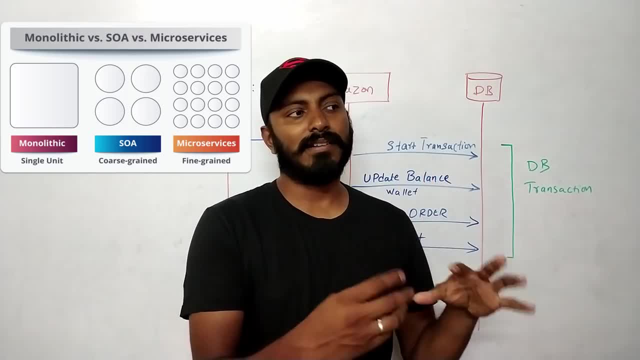 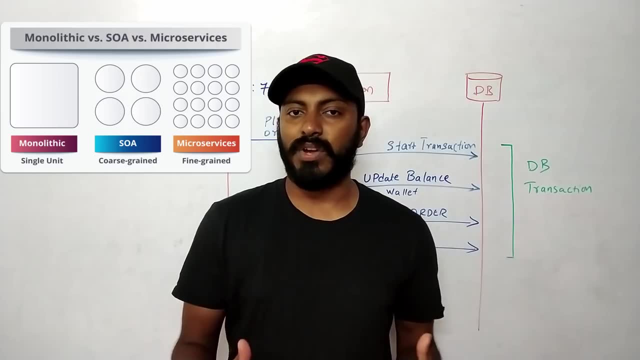 are bundled into one specific service and that itself can be scaled independently. Whereas in micro service architecture is a different variation of service-oriented architecture in which you basically the application is made of small, you know, independent or loosely coupled services To understand transactions in micro services or transaction in distributed systems. 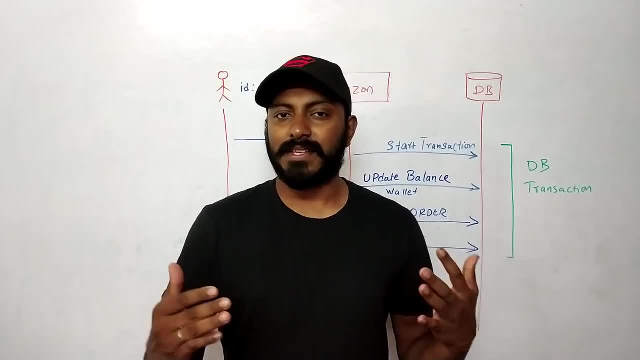 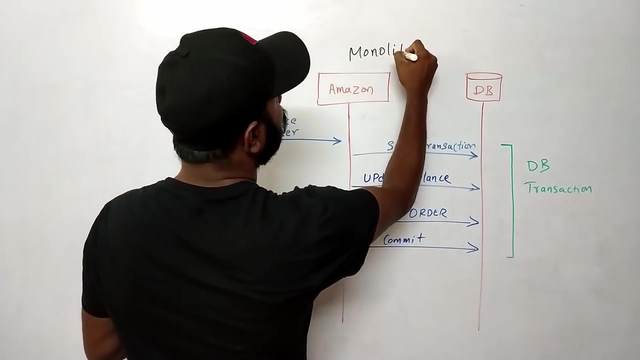 we need to take couple of examples and then see how it used to behave in monolithic architecture and then how it behaves in micro service architecture to understand it better. So I have an example here. So this is the architecture for monolithic. So this example is from monolithic architecture in which the user is trying to place an order. 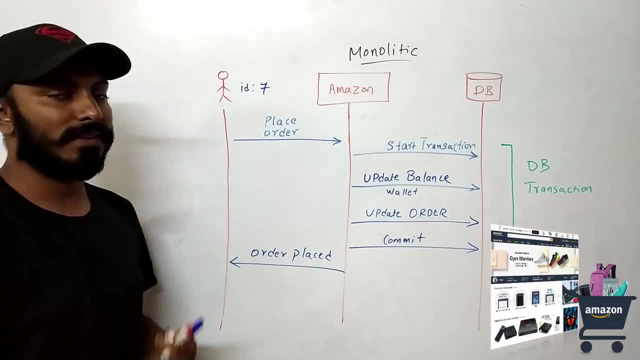 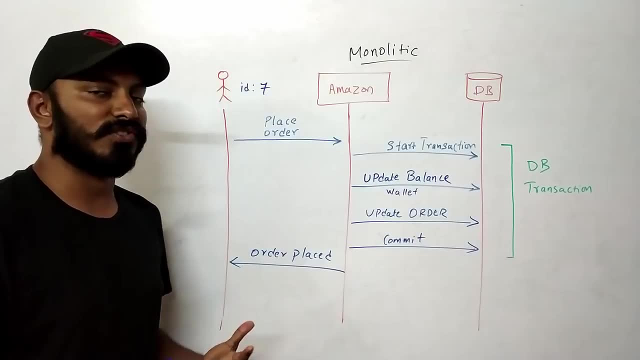 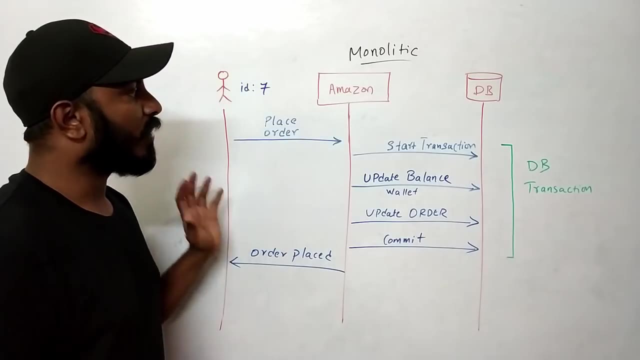 at Amazon website by paying some money which he has in his wallet. So we are interested in transactions. right, because the video is all about distributed transaction. In case of monolithic, it is not really distributed at all because we have one service which is basically the Amazon website itself. So all of the services 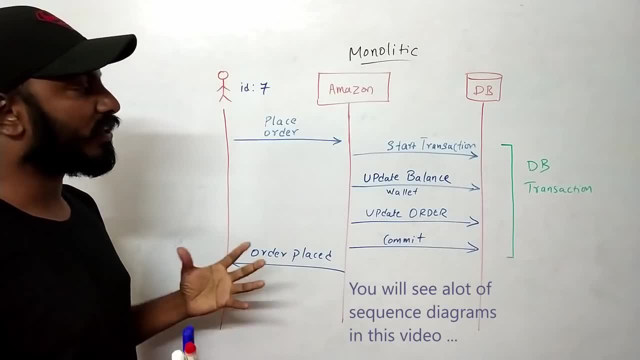 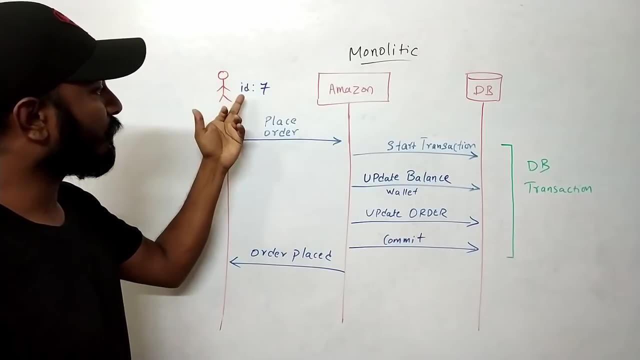 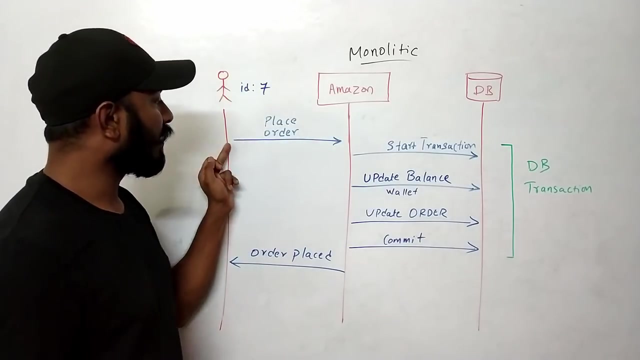 connected to one database. This particular user is trying to place an order. So what happens? The sequence diagram will explain that. So when the user maybe, for example, take item with seven places an order at amazoncom, some order, So you'll make a call to Amazon service. 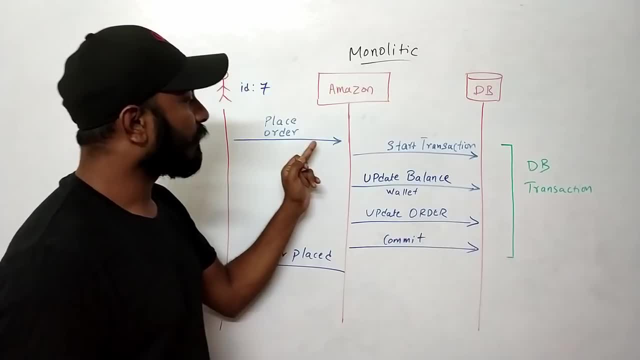 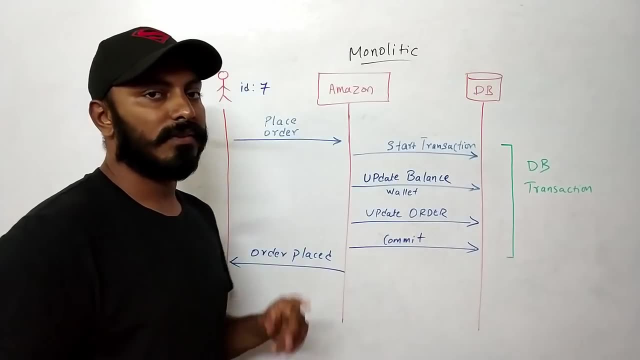 and this is whole of monolithic service. and then this service is going to start a transaction and does two important actions. To successfully place an order, he has to first check the balance and update the balance by deducting the price of the product, and then he has to place the order. 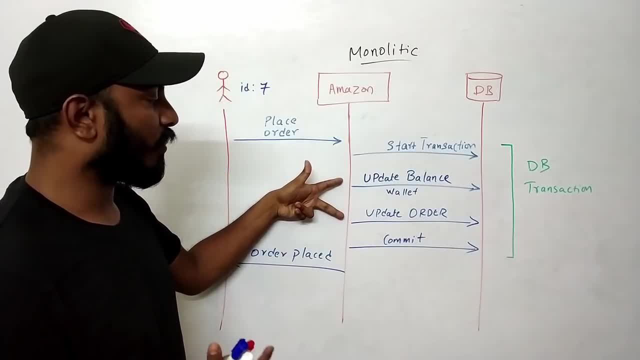 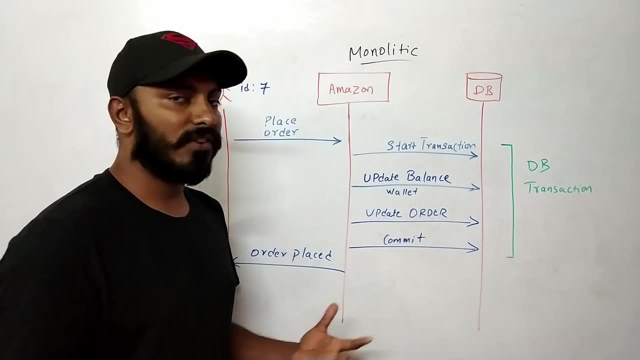 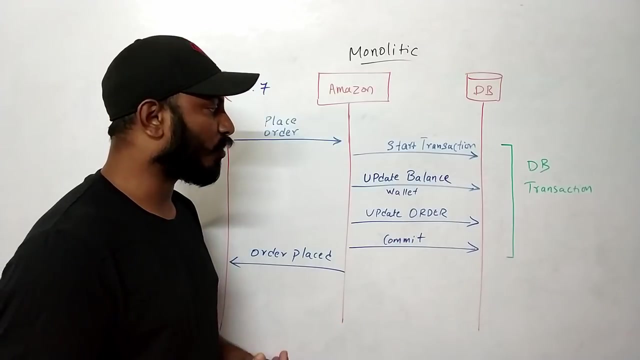 There are. so these are the two important you know queries which is actually happening. So, before doing that, as you learned from previous you know videos- that we need to have a transaction because we have to treat these two queries like it could be select, or it could be update or it could be insert. has one single unit of work. 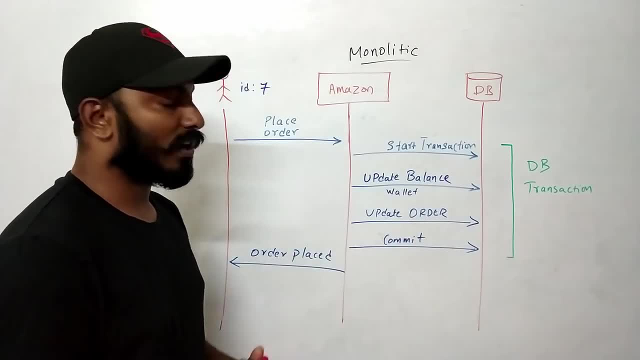 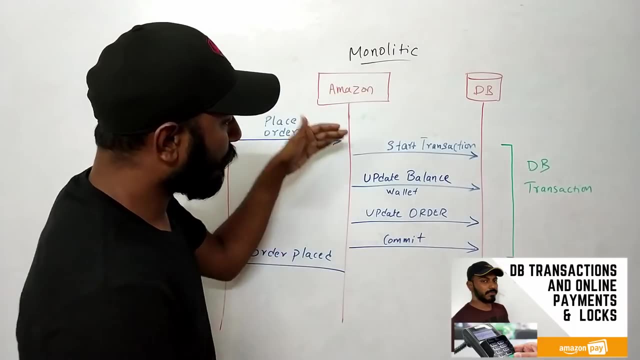 to make all of this process atomic. Otherwise there are a lot of problems which happens. Please refer to the other videos which I have made. So we have put all of this into a transaction so you can see I've referred it as DB transaction. So first, 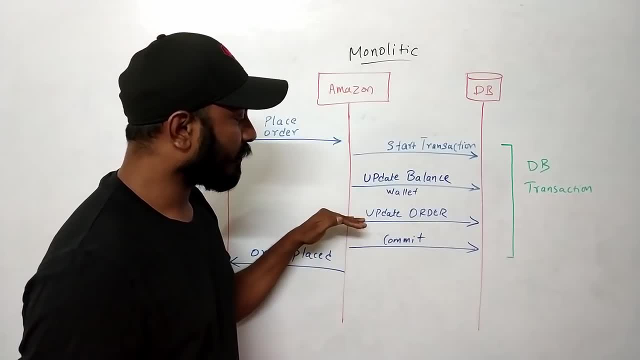 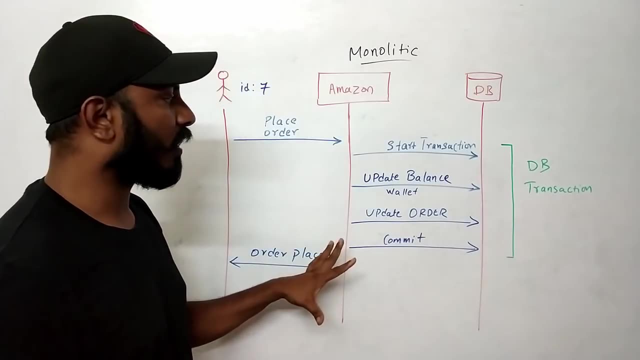 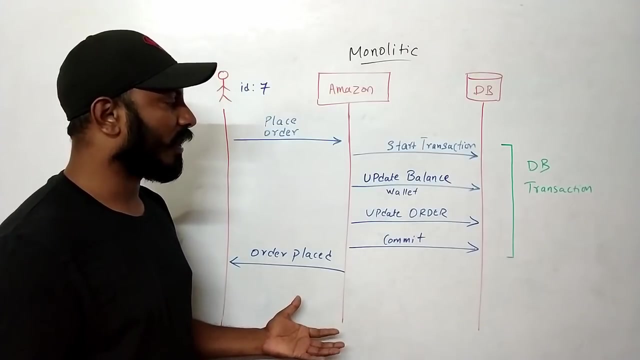 what we do is update balance in the wallet and then second place an order or update an order into the database. So this works smoothly. because it is a monolithic architecture, nothing is going to go wrong because we have isolation. it's completely atomic, So everything works fine. 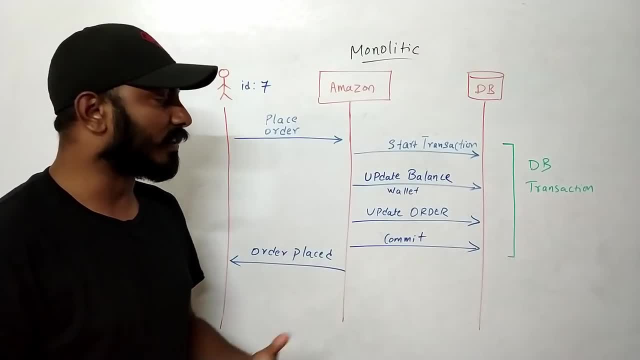 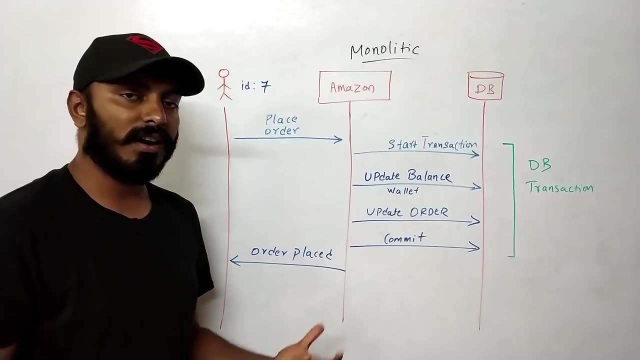 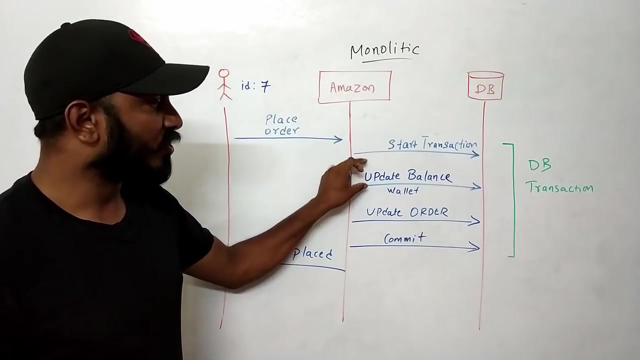 Suppose what happens if the user doesn't have sufficient balance in his wallet. So this is the step where we are basically updating the balance, the wallet. that's where we actually check whether he has the balance in his wallet or not. In that case, this query will definitely fail, so we basically does nothing. So because of the transaction, 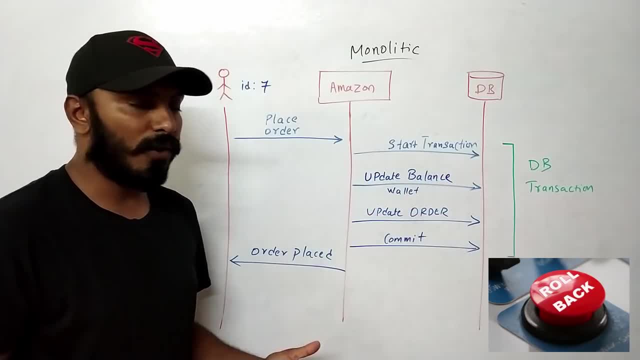 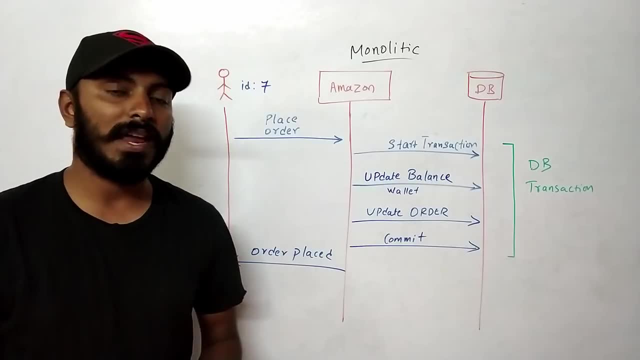 every previous action will basically will be rolled out and we basically doesn't commit, so nothing is going to happen. Basically, the user will see an error showing that you don't have sufficient balance. So what if he has a sufficient balance but we don't have enough products in our 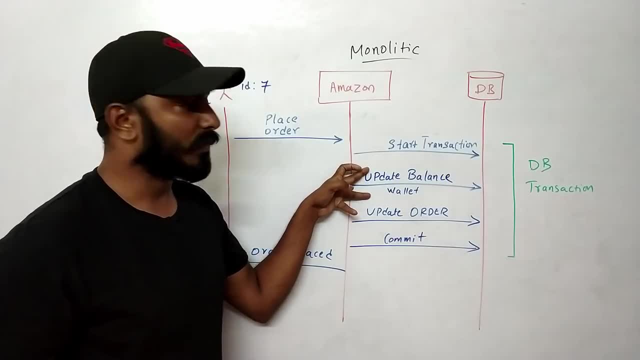 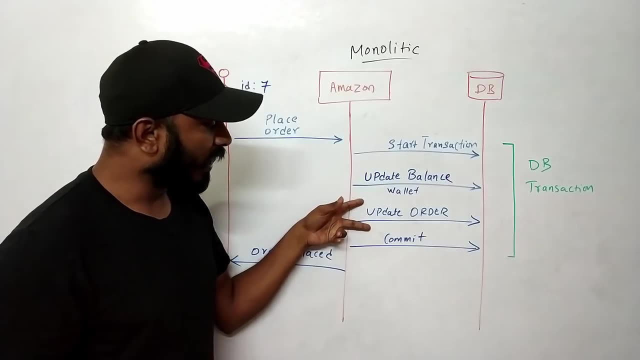 inventory. So in that case we will update the balance. Remember, we haven't committed yet. We will definitely update the balance by deducting the amount he was supposed to pay, and then we will try to place an order and we see that we don't have enough product in the inventory. So 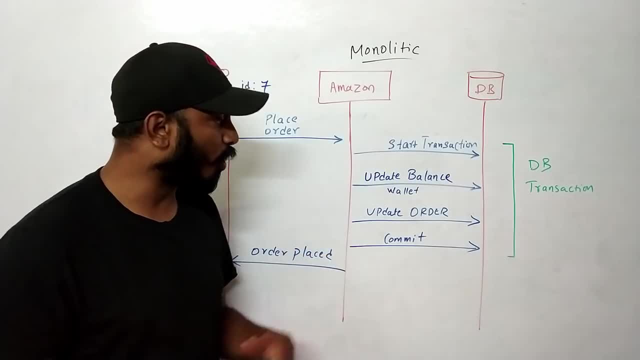 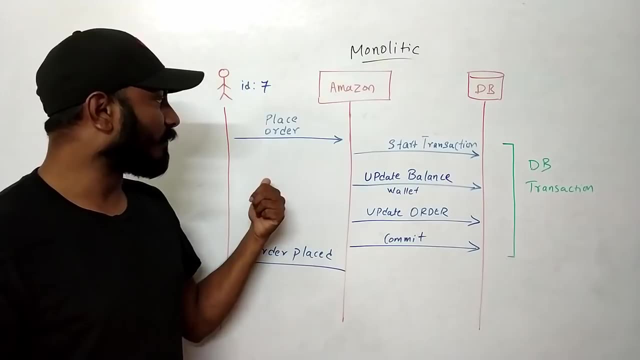 this particular query will fail and we don't commit and we basically roll back. So all the deducted amount will be put it back to the in his wallet and then again a user will see an error showing that we don't have the product in the inventory. 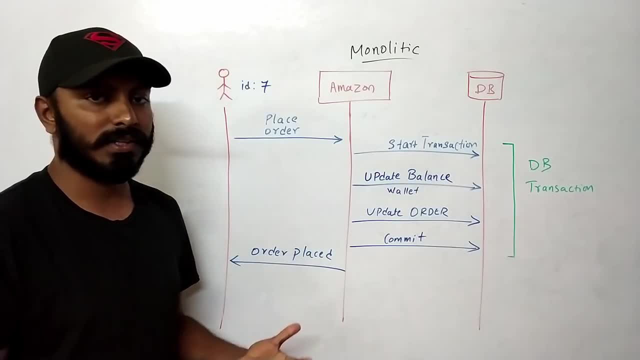 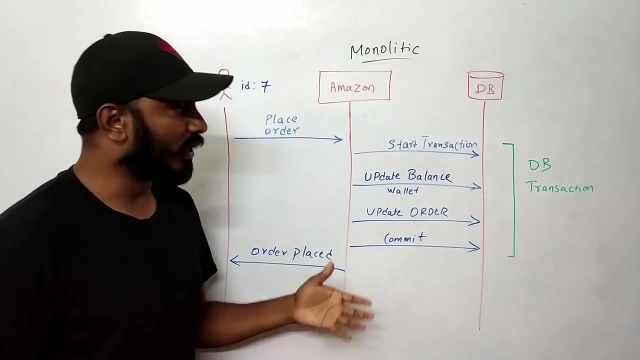 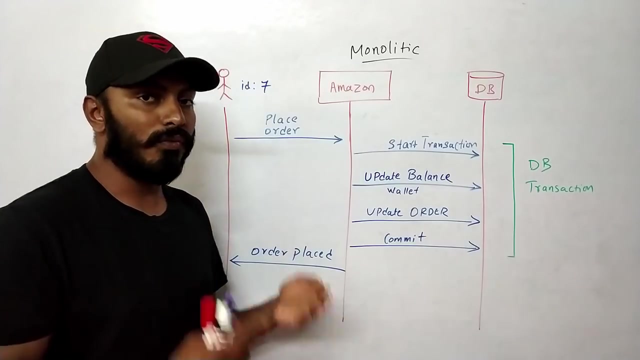 Please check back later. So that's how it is protected, Even if two or three- you know- parallel transactions are going with the same user ID. but still, since we have started the transaction, that particular row will be kind of locked, so other transaction will be waiting until this transaction. 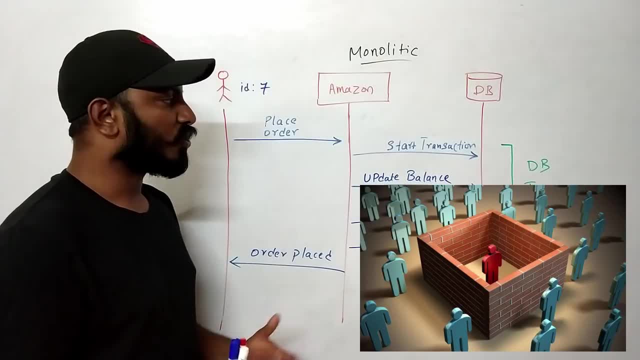 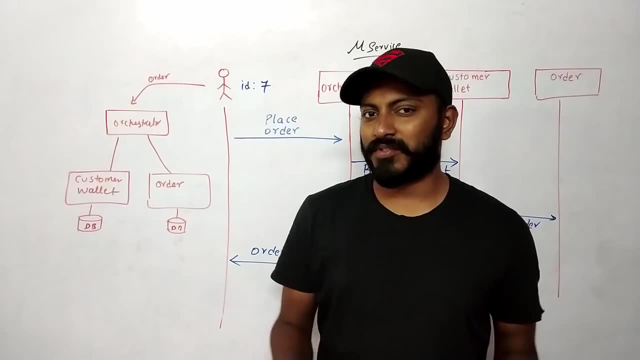 releases the lock, so the isolation is provided. So what happens in case of microservice? How do we do the same transaction in microservice? And now we have the microservice, Now we have the microservice architecture for the same example and, as I told you, this is loosely coupled services, basically the 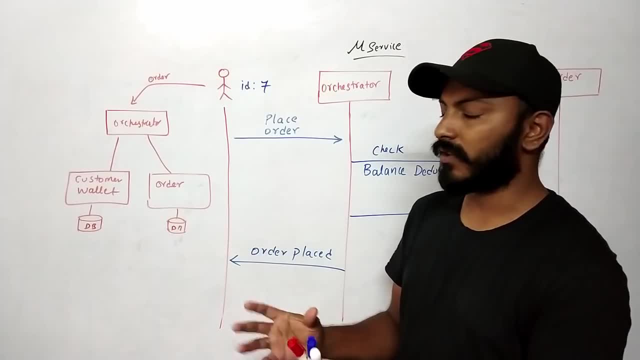 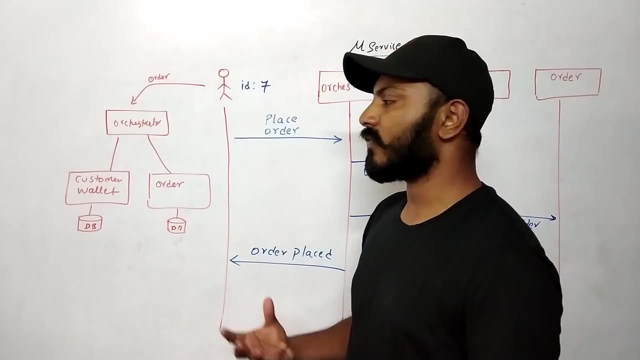 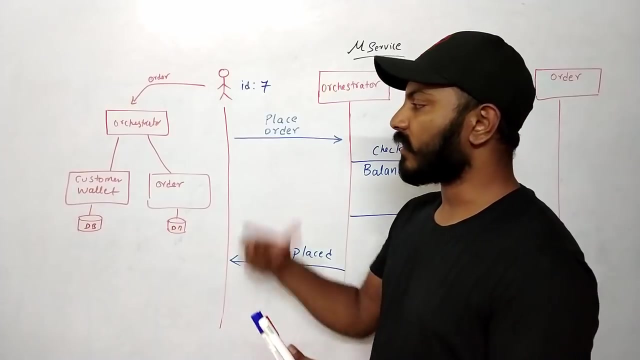 small services which are which makes up a complete service or complete application. So in this case the same application has orchestrator, basically that's the one which basically receives the call from the user and then fires so many calls and then collects the results and give it back to. 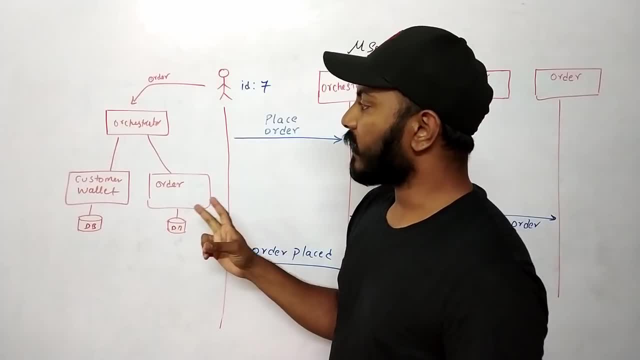 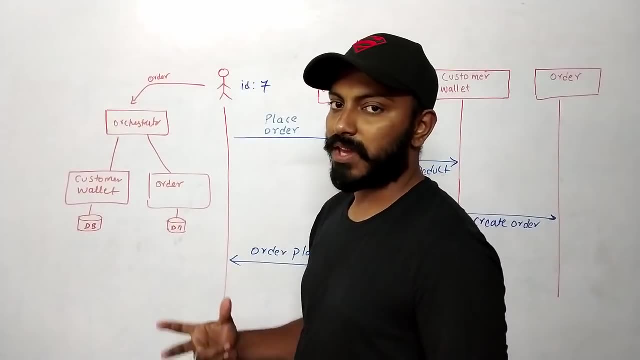 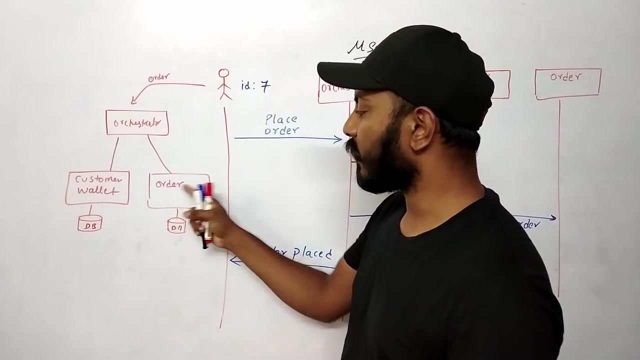 the users or the API calls. So in this case, whenever user places order, basically the orchestrator calls two different API calls of microservices. and now we have two microservices for this purpose. One is customer wallet microservices and the other one is order microservices, and they both have their own databases. They are not sharing their database. 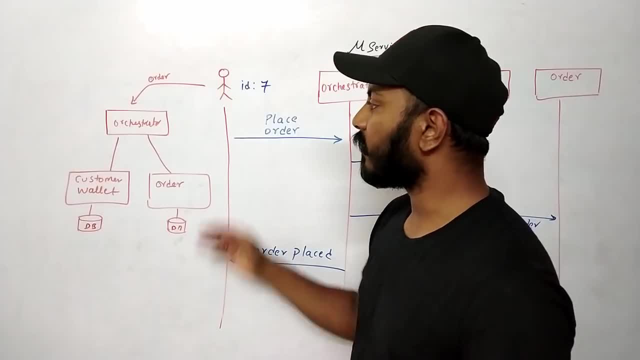 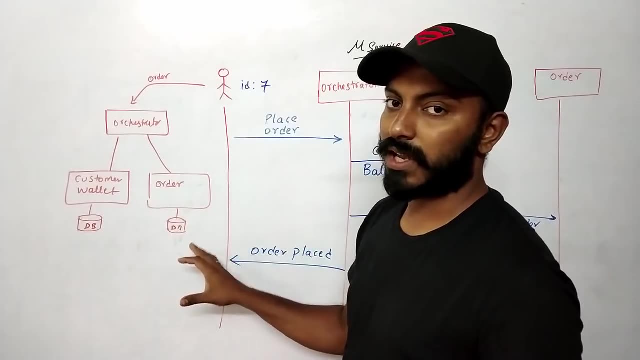 Okay, so now whenever the user wants to place order, he makes a call to orchestrator and orchestrator fires request to customer wallet and order and then the process would take care. And let's see the sequence diagram: how exactly it happens. Now the same customer with ID7 places. 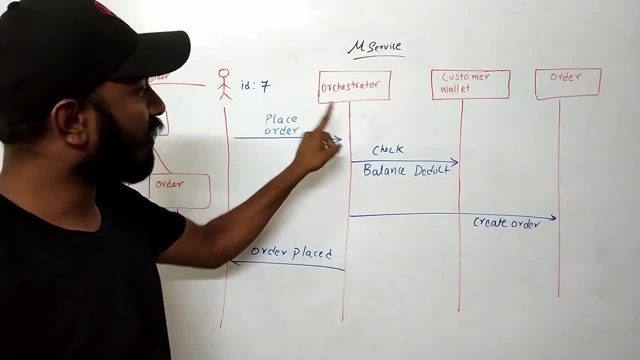 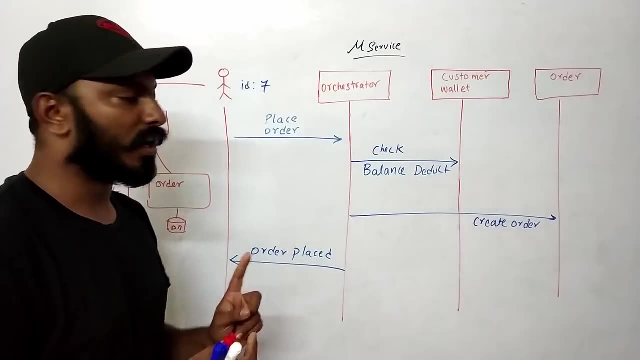 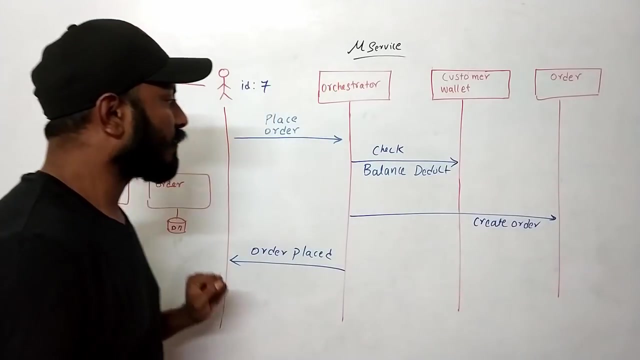 an order and the orchestrator receives that call. and then the orchestrator basically makes two calls: One for customer wallet, because he needs to deduct the amount, and then he also needs to make a call to place an order or create an order to the order microservice. So now, what he does? he does either 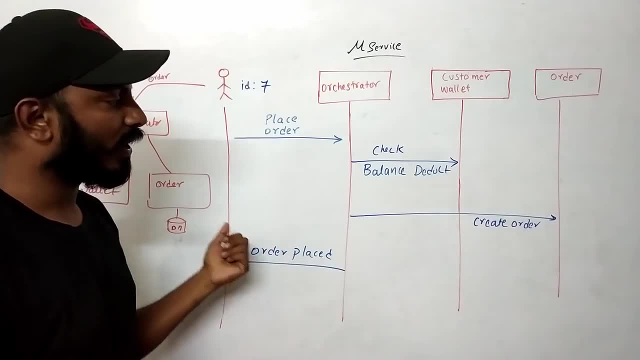 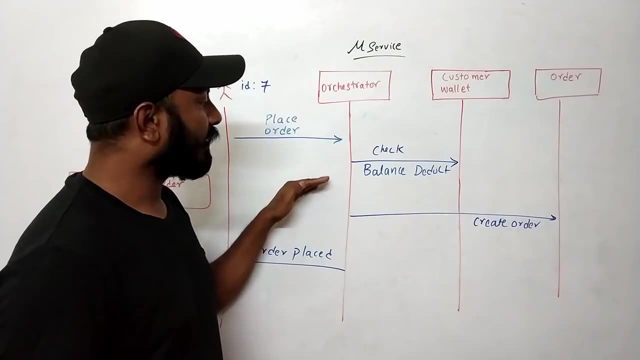 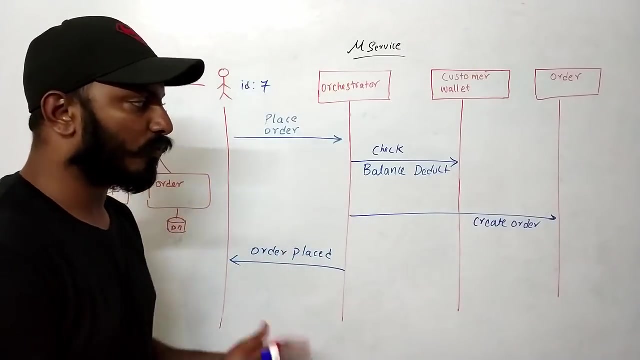 fire. those calls one after one or in parallel. So let's consider one after one. So first it makes a call to deduct the balance and then he makes a call to create an order. So do you think this will work? This will definitely won't work, because the 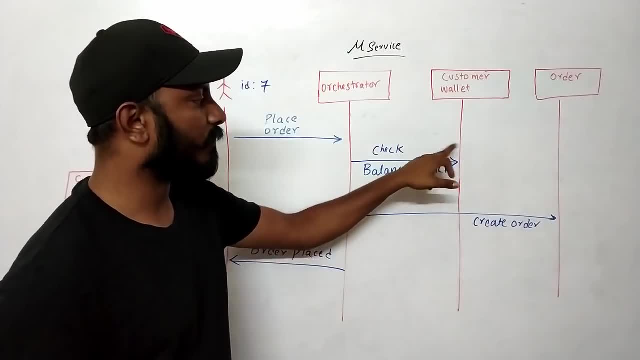 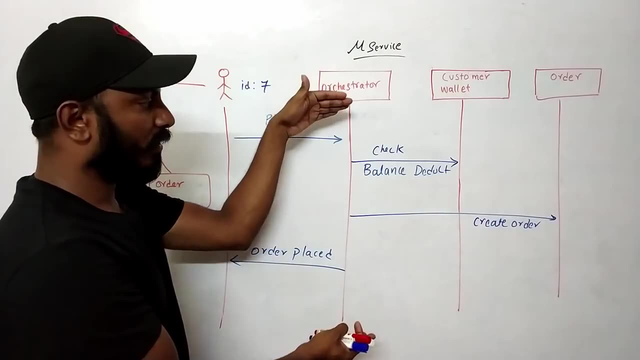 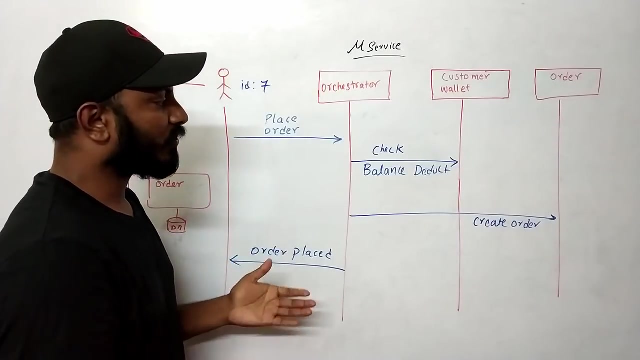 transactions are limited to their own, you know local or individual calls of that particular microservices. The transaction is not kind of global usually in if you see the monolithic, the earlier sequence diagram, where in monolithic we had the transaction for both of these kind of queries Since the 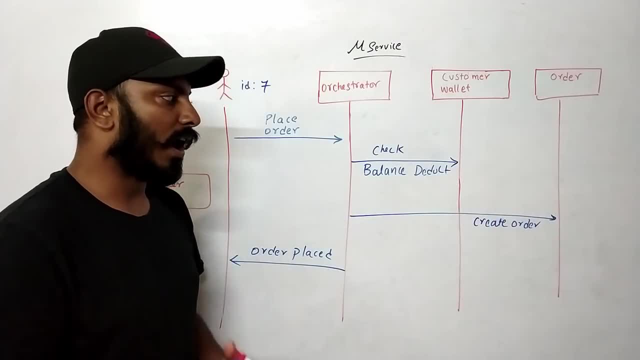 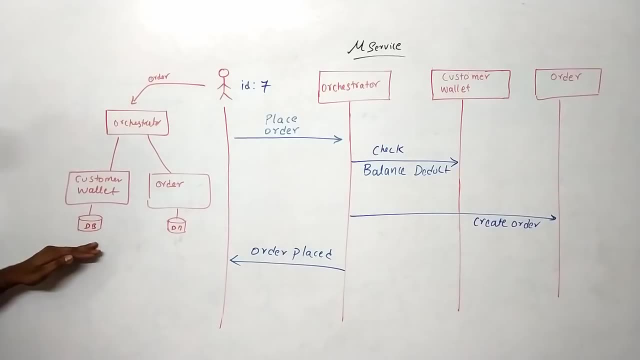 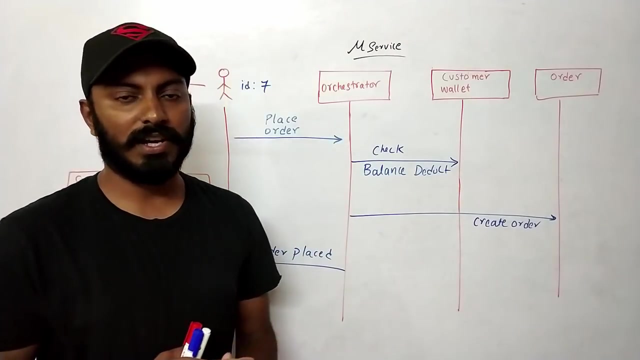 services are split into small, small services individually. now we can't have this one transaction for both of the calls, because these two services are not sharing the database, because they have their own databases, because that's how microservices are built. So now the isolation is not, definitely not there, because when you, when this first call happens, he will deduct the amount. 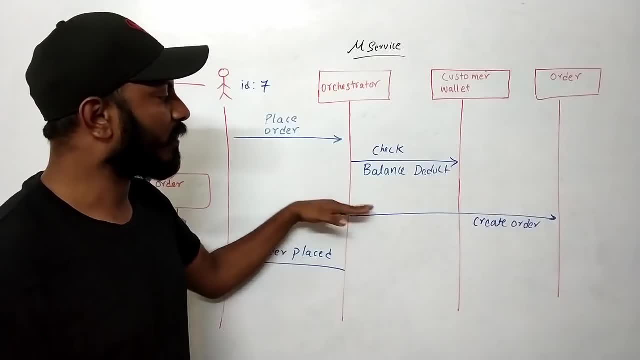 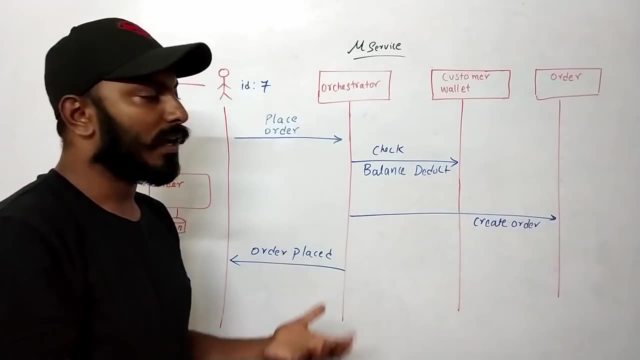 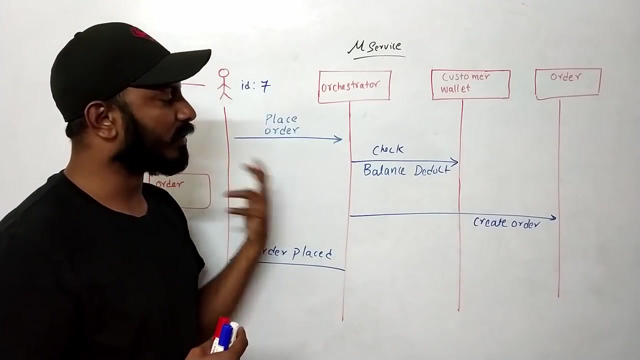 and then the create order will call will happen By the time. what if one more my call for the same user gets into here and he sees the directed balance? basically, still we haven't placed the order, but already the users. the user is seeing the deducted balance and the order is still not placed. So these 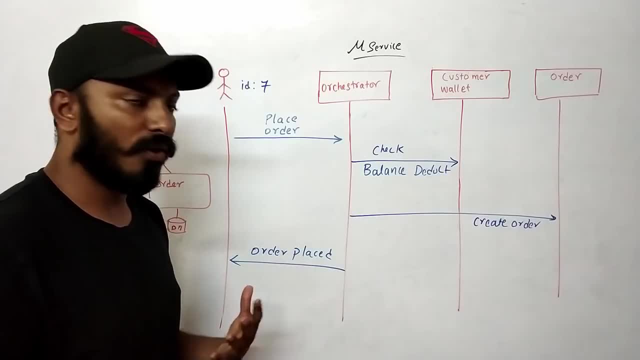 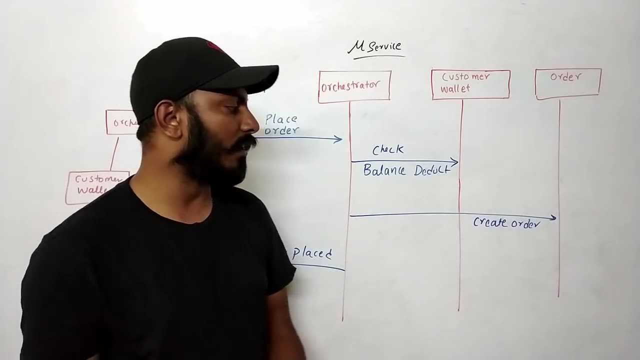 kind of problems are there? What if this fails? what if this fails? and who will take care of the failure scenarios? What if the balance was deducted and then the order is failed Because we didn't have enough? you know products in our inventory, So who will take care of you? 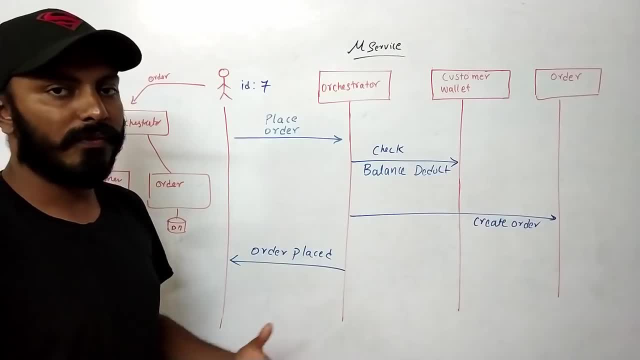 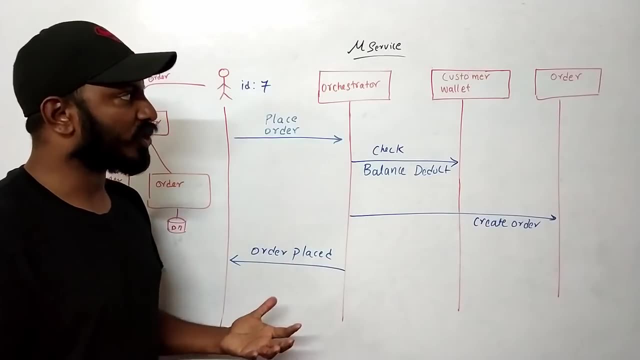 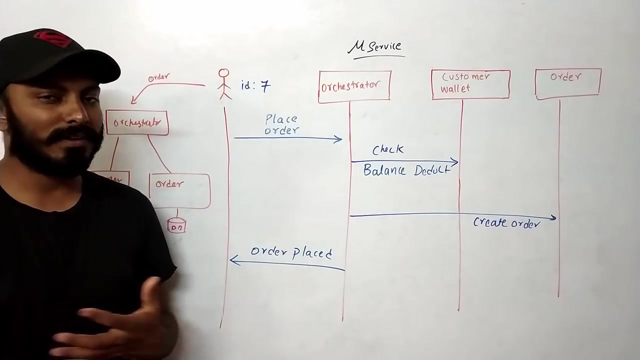 know, rolling back the amount, whatever we deducted. So this is all a little getting messed up. So how do we solve this particular problem of transactions in microservices? The concept to solve this is called as distributed transactions, and there are so many algorithms, or you know the process to make. 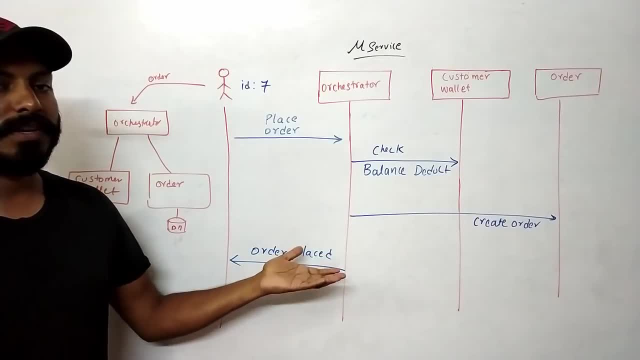 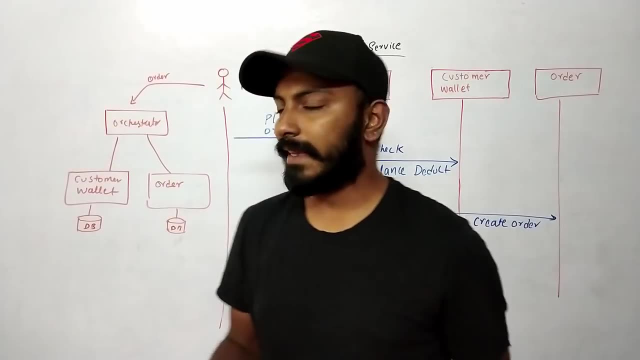 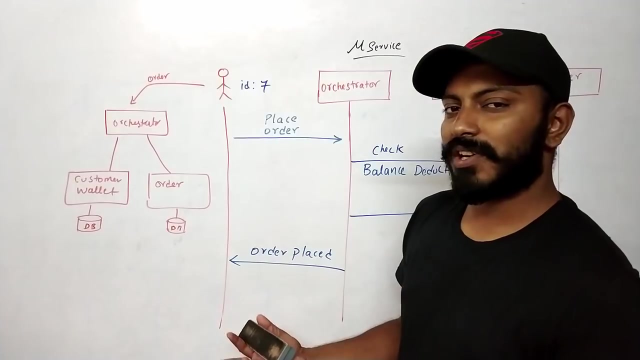 sure the transactions work in distributed systems. So, before solving that here is a little crazy idea. So, instead of doing anything, can we do something to this microservice and solve this particular problem? So, yes, actually we can, right, because, see, instead of having two different databases for these two services, because 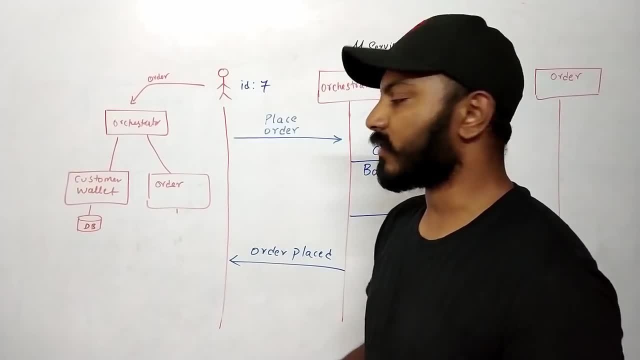 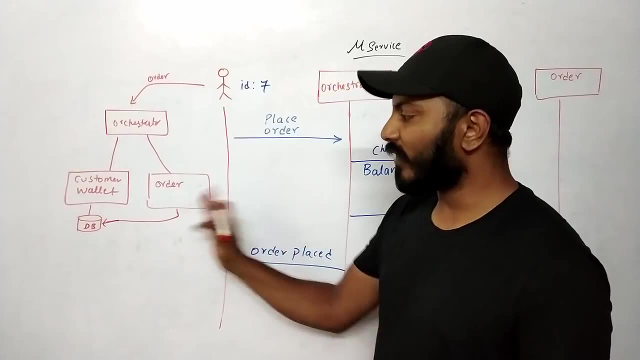 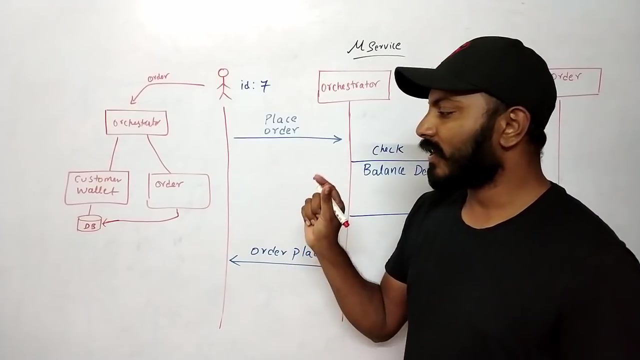 we know that these two services are kind of dependent and we need a transaction. why don't we just connect order and customer wallet to the same database? So will this work? Definitely, if you work, because these two are services and they both are connected to database and they should work. But this is not the ideal way of building. 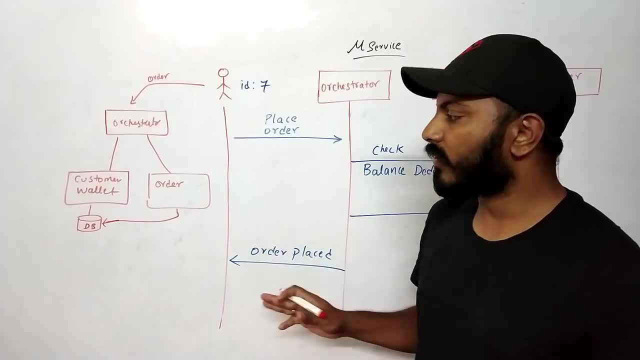 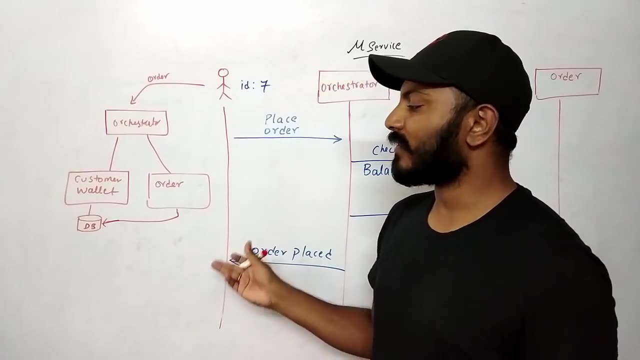 microservices, because this is anti-pattern, where two different services shouldn't be connected to the same database. Instead, a couple of guys have, you know, you know a couple of guys have violated and still go ahead and do it. but it's fine, but it's not really scalable and this is not the 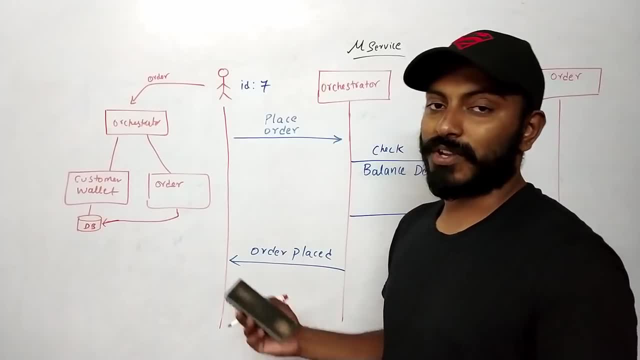 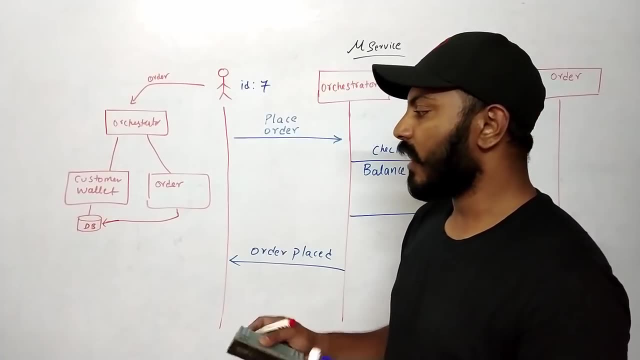 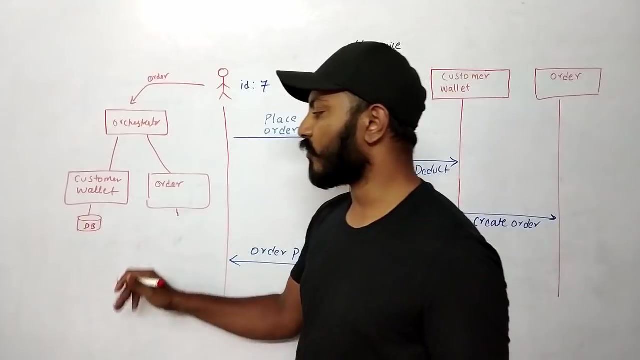 reliable way of doing it. I mean, of course, you can do whatever you would like. end of the day, the solution should be neat and it should be reliable and should be scalable and all of that. So the other techniques. what people recommend is, instead of having you know, two services connected to the same DB have a. 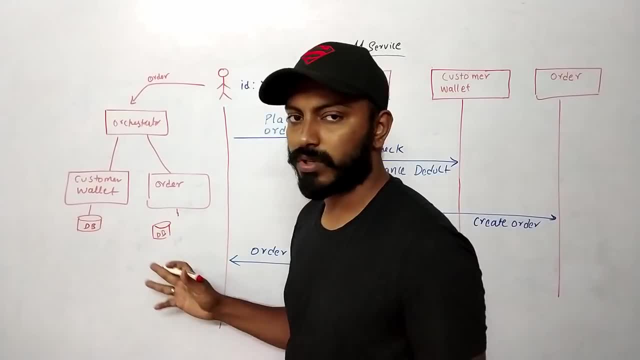 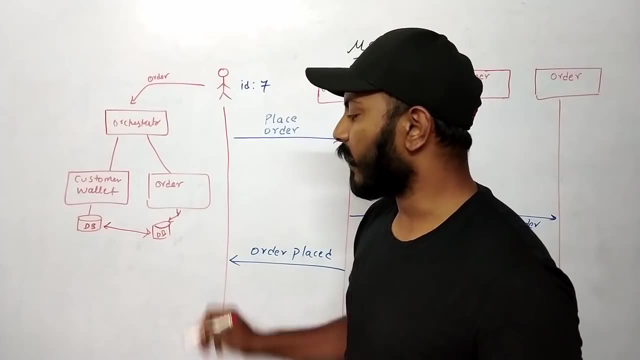 replication strategy of you know, kind of like, you have the two different instances of DB and they both are replicating the data between each other and this is, you know, still fine. but the only problem you see here is because of the replication. the consistency goes for a truss In this. 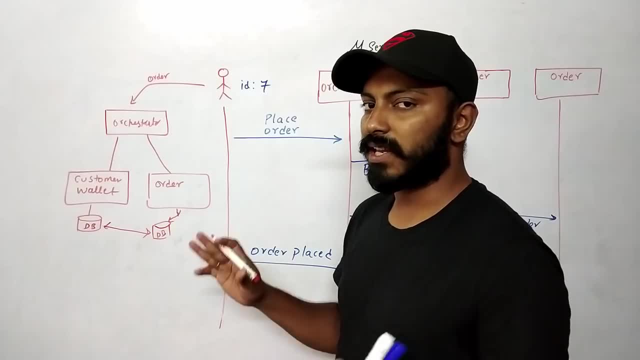 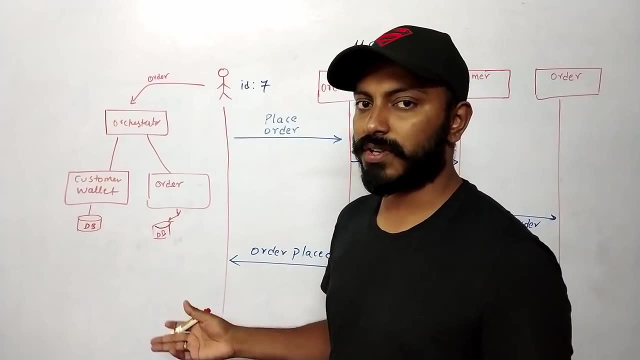 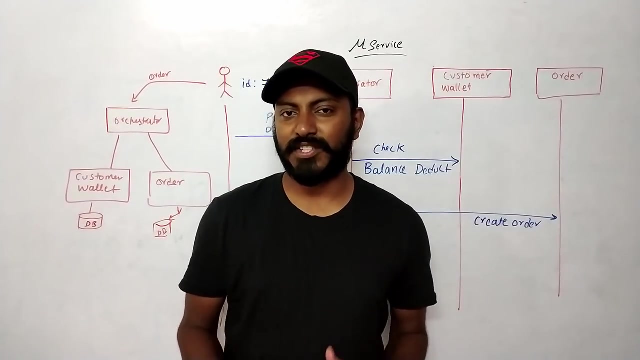 system, the consistency will not be there. If your system doesn't need consistency, then you can do it this way. otherwise you will have to stick with having individual databases and you should still implement the distributed transactions for microservices. So how do we really solve the distributed transactions problem? The answer is two-phase commits. 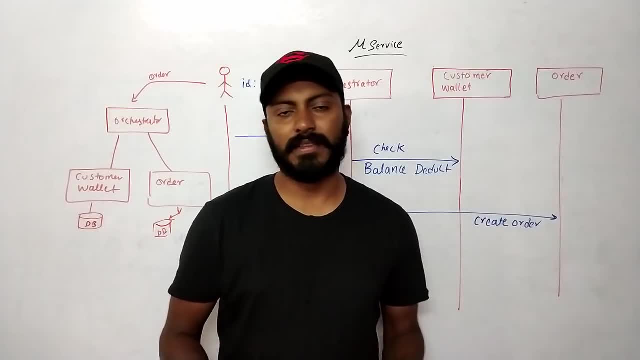 Saga. So let's learn the phase commit first and then we'll concentrate more on Saga. So there are so many people who have implemented two-phase commits in a lot of different projects and everyone has their own different opinion. Some say two-phase commit is not really good for microservices. Some say it. 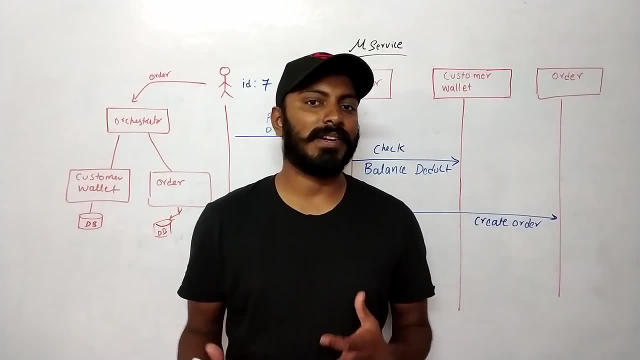 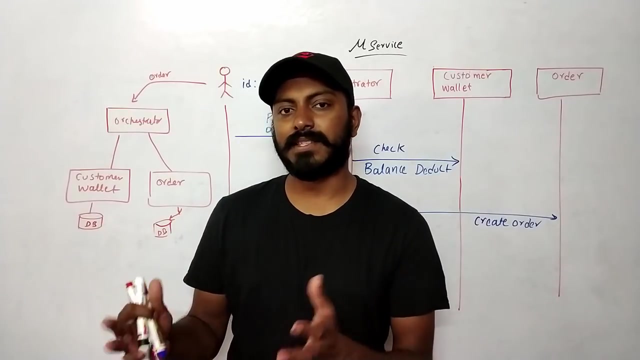 all depends on the use cases. Personally, I haven't implemented on my projects. This is all the information I was able to collect from different blogs and sites, So I'm not going to recommend what to do, but this is how we can actually solve the problems, If it really fits to your use case. 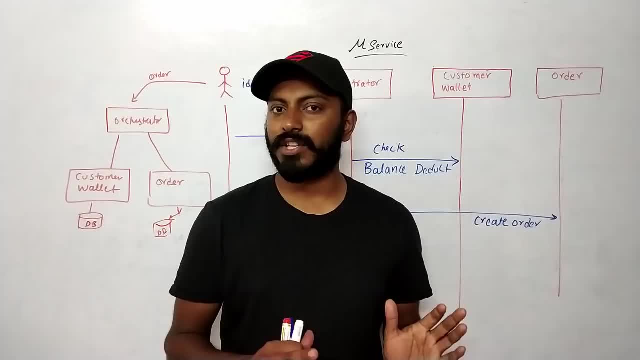 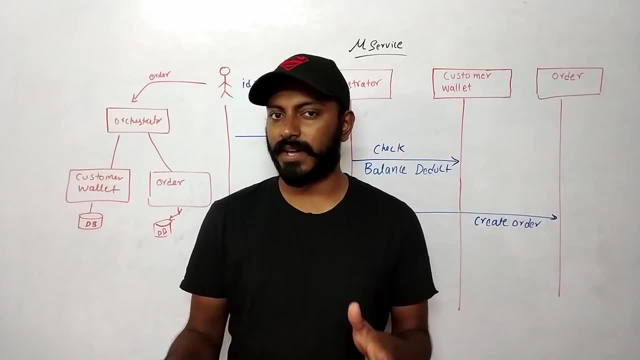 definitely go ahead and implement it. If it doesn't fit it, use a different way of implementation. Maybe Saga will definitely help you. If you think two-phase commit helps you, then please go ahead and implement it Now. let's understand what is two-phase commit. 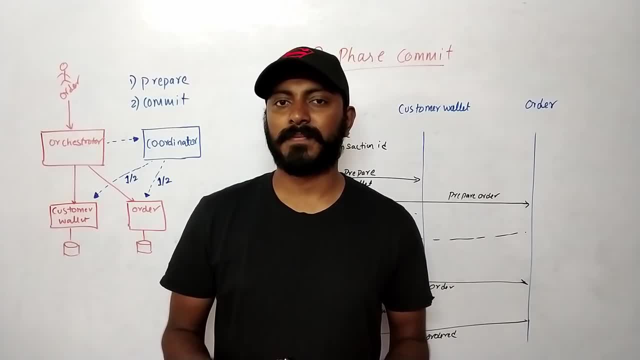 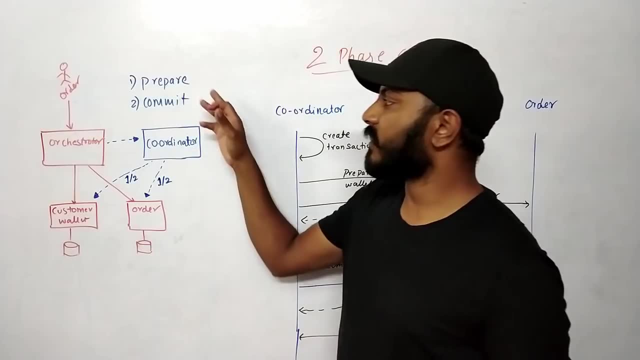 With two-phase commit, we choose two phases of operation, As in the name it has two phases. That means that we have two phases to do it. So the first one is prepare and the second one is commit. Basically, who tells you to prepare or commit? 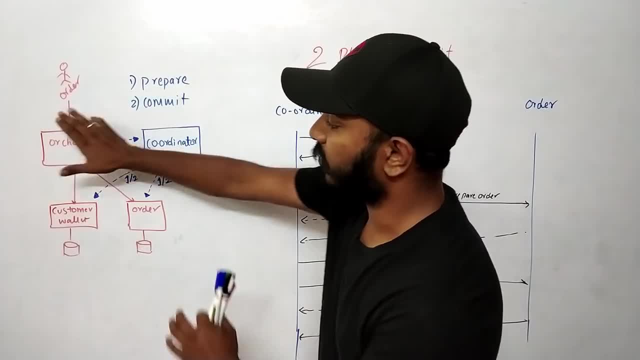 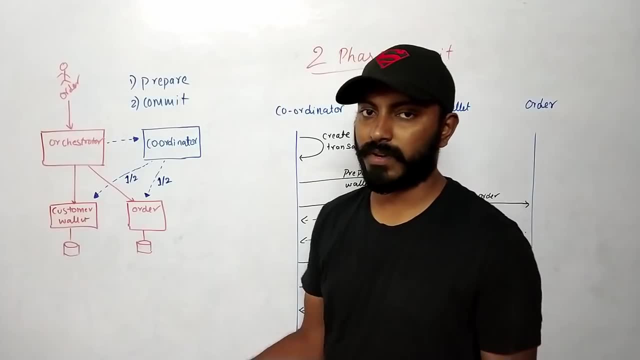 So, if you remember, in the earlier diagram we had this much, right, We had this much, We had Orchestrator, we had Customer Wallet Microservice and Arda Microservice and we had two different databases which are connected to individual services. 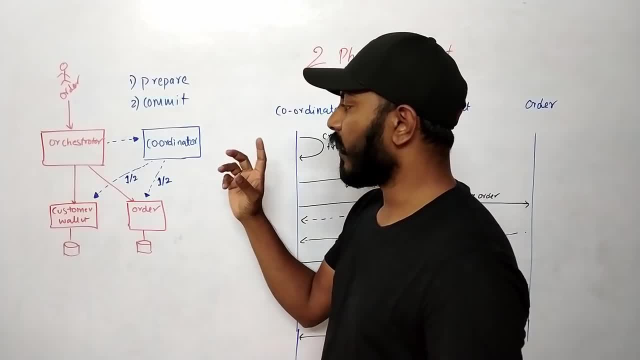 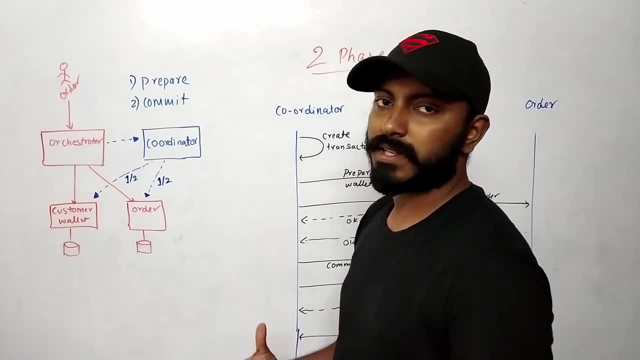 So to understand how two-phase commit works, we have two phases. First we have Arda Microservices and we have two different databases Which are connected to individual services. now we have introduced one new server or a component called as coordinator. now for this, for the sake of simplicity, i've written it as separate one. but in real world, 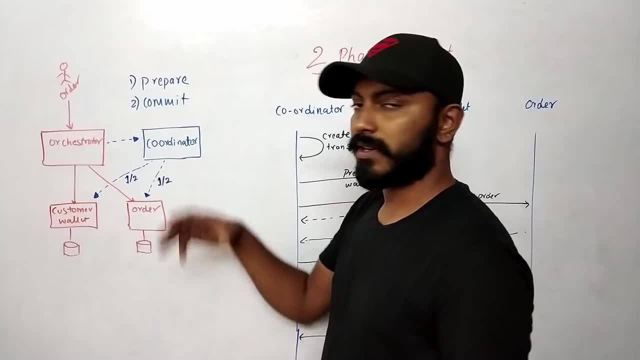 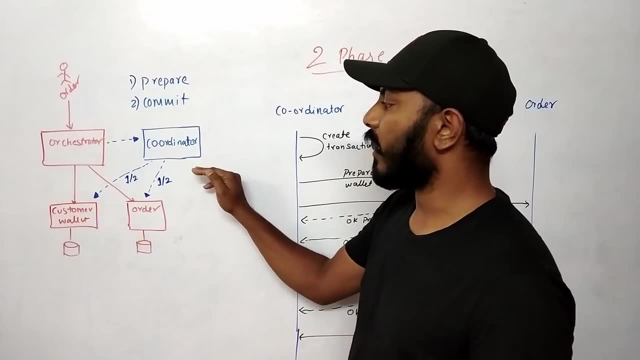 this could be present in any microservice, or it could be an independent service itself, so let's keep that as independent services. so what this coordinator does is this is the one who actually takes care of two-phase commit. so in case of any other commits- uh, like a layer. 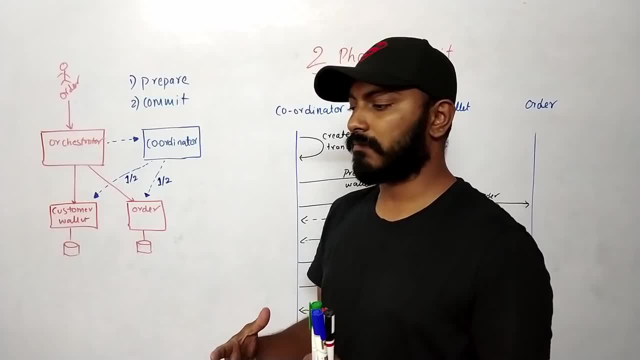 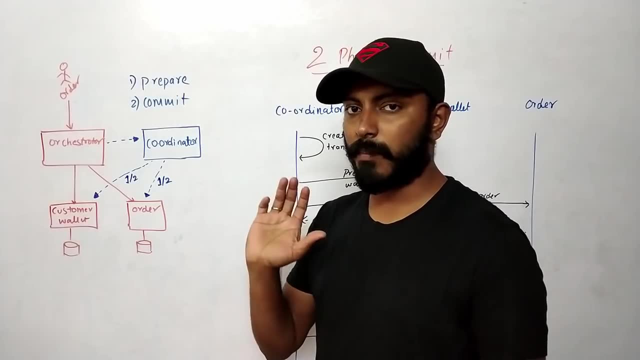 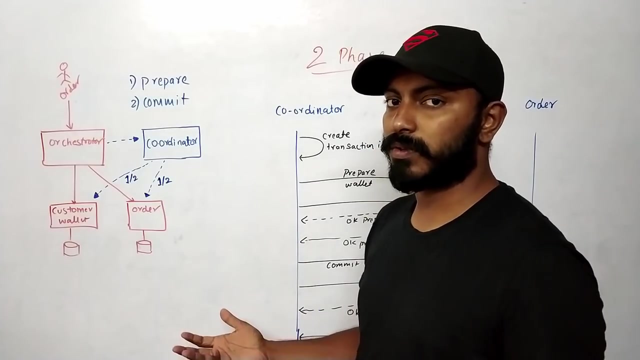 transaction. commit. they are all kind of like: um, not exactly one phase. commit, they are like, uh, it's just one entity, right, so any commit happens, it happens at one shot, but in this case the commits won't happen at once. basically, it has two steps to do commit. one is prepare and one is 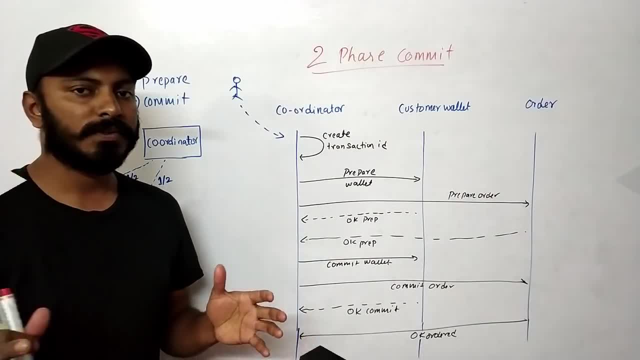 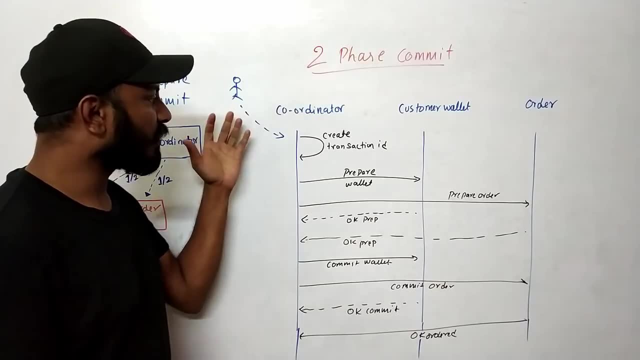 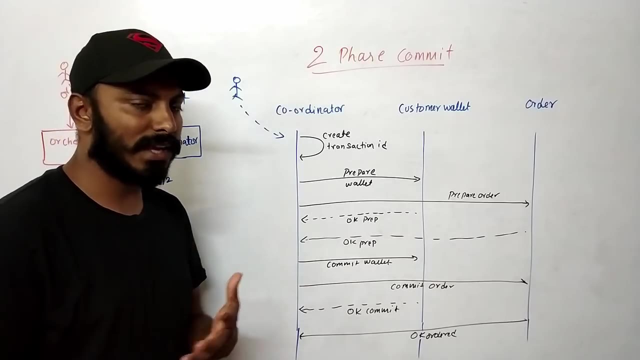 coming, so how this exactly works. so let's see what happens when the user places an order to the system in the form of sequential diagram. so when the user places an order, the first thing will happen is the coordinator should first create the transaction id, because that's the id which will be referenced to, or given as a reference to all of the different 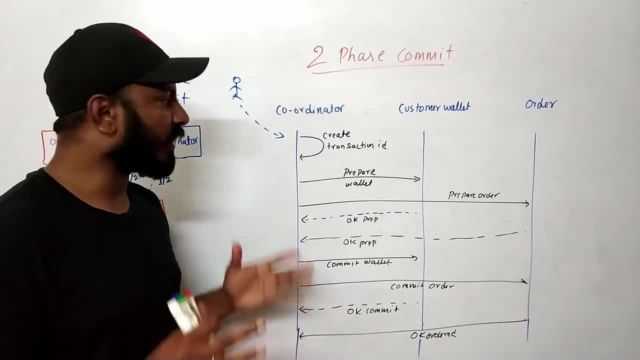 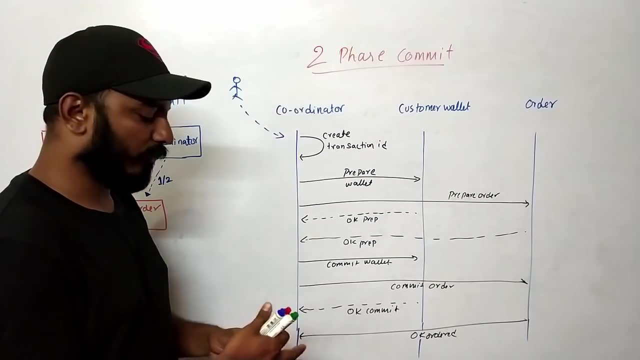 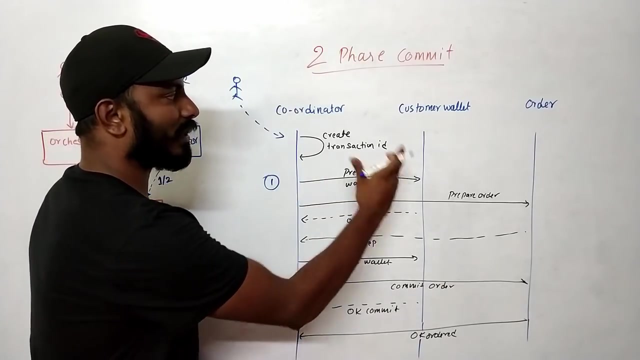 microservices which the coordinator is going to talk. the first thing the coordinator does is the prepare phase and then the commit phase. so first he has to do the prepare phase. in this case that's the first stage, right? so in this stage the coordinator will ask the customer wallet and also 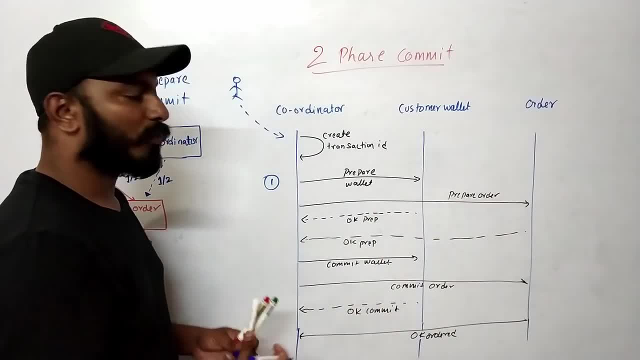 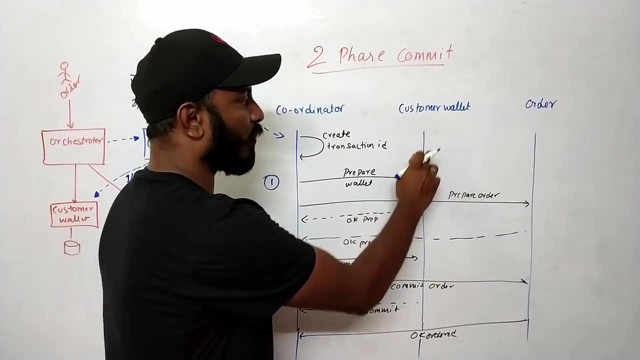 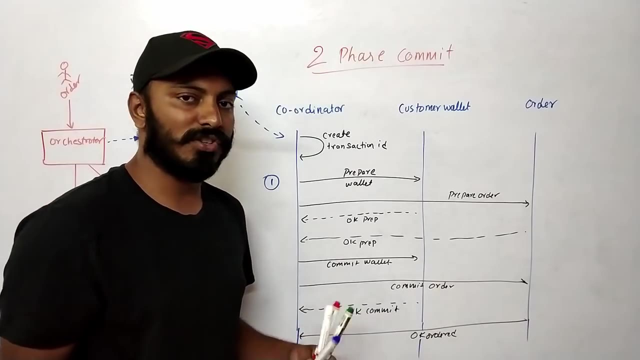 the order um microservices to prepare their states. what that means is basically: when coordinator asks the customer wallet microservice to prepare what he does, is he basically checks for the balance? does the customer has the balance or not? if he has it, he basically locks that uh particular. 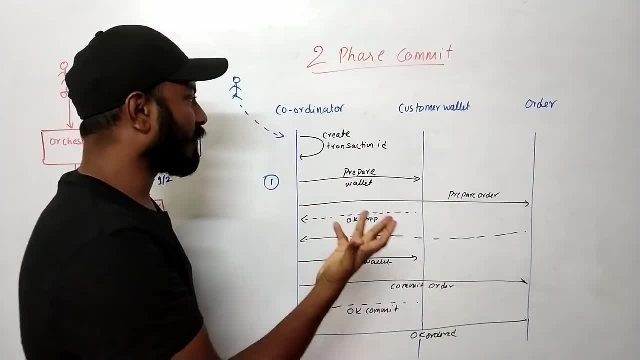 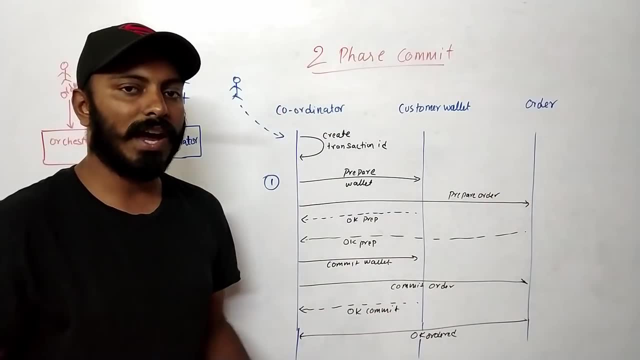 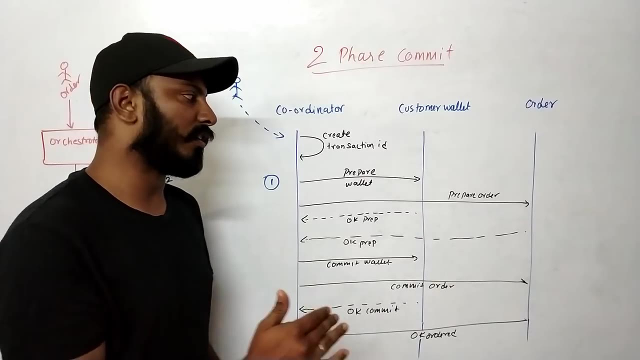 order using the transaction. okay, and then the same thing happens um with the coordinator. when, when the coordinator talks to the order of microservices as well, he will basically check if that particular order exists um in the inventory or not. if it is, it will basically block that particular order for himself, and then both of the services basically reply to the coordinator. 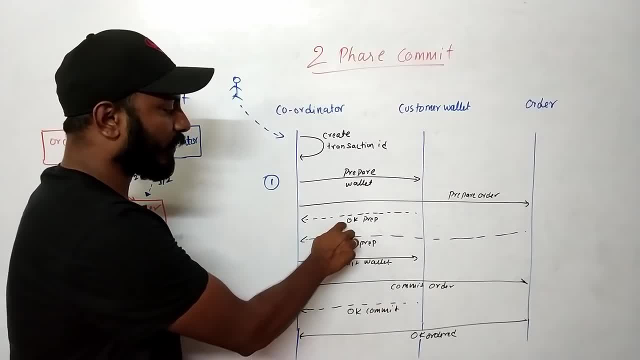 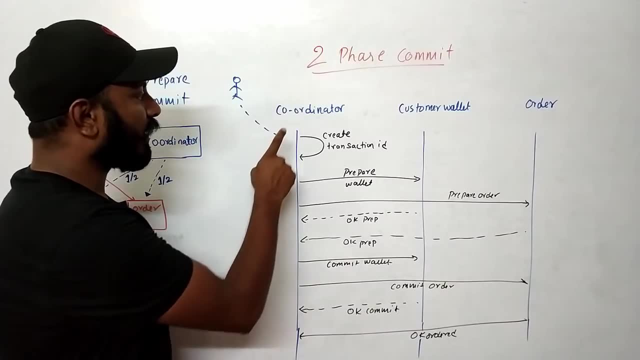 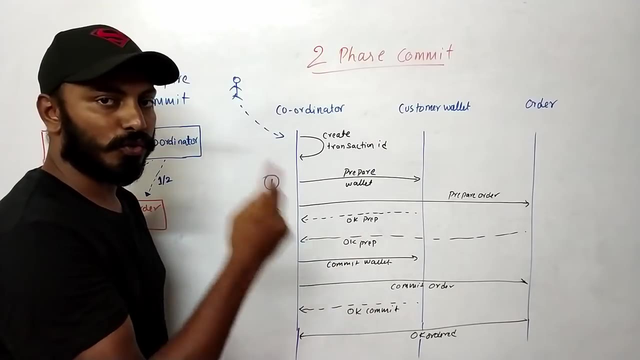 that, yeah, okay, we have prepared. so this is the call which basically says that we have prepared by the and also by the order, that, okay, have prepared the order. so now the coordinator will be basically waiting for two different calls because it knows that i have made a request to two microservices: one: 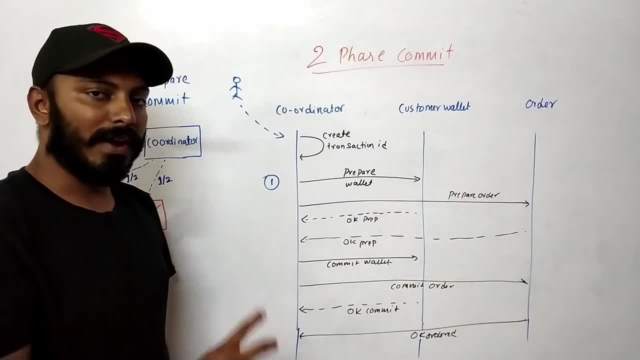 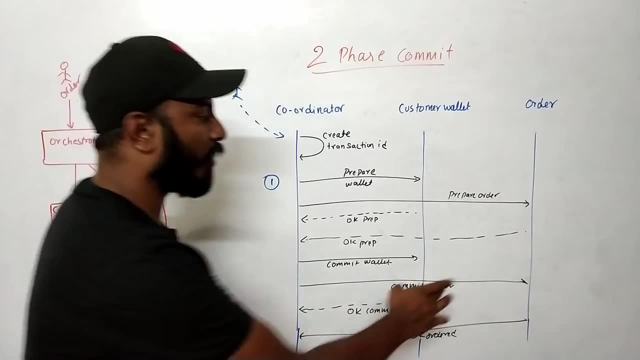 is customer, one is order, microservices. so he will be waiting until um two callbacks or two responses. if, for example, if the order response took some time to reply, then the coordinator will not do anything. um, then the coordinator will not do anything. um, then the coordinator will not do anything um. 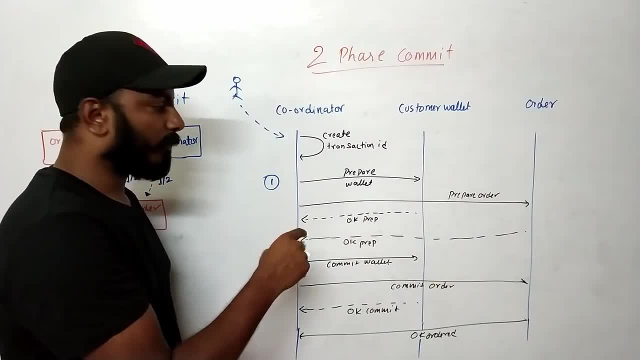 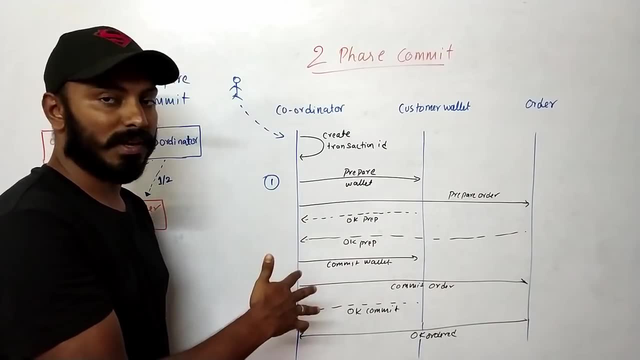 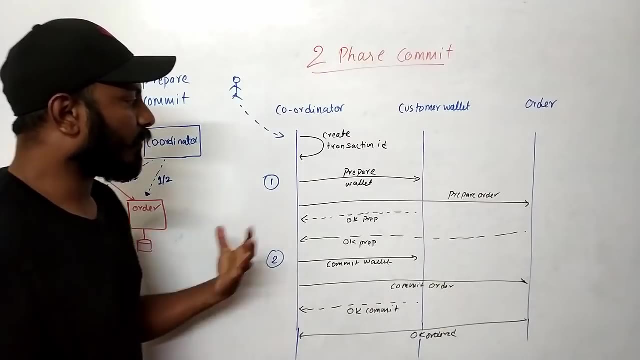 but wait, uh, as soon as he gets um two calls, he will basically continue with the second uh phase of the you know uh two-phase commit. the second phase of the two-phase commit is commit. so in this case, um once successfully prepared, the coordinator basically asks the: 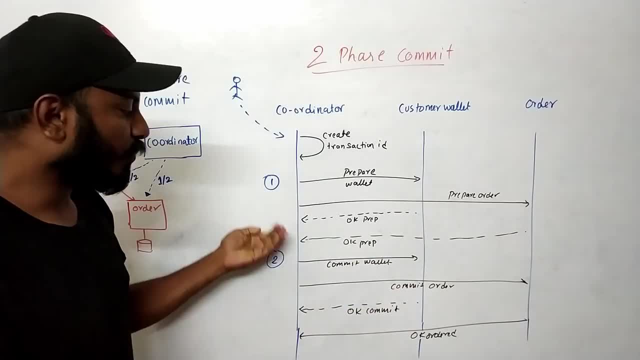 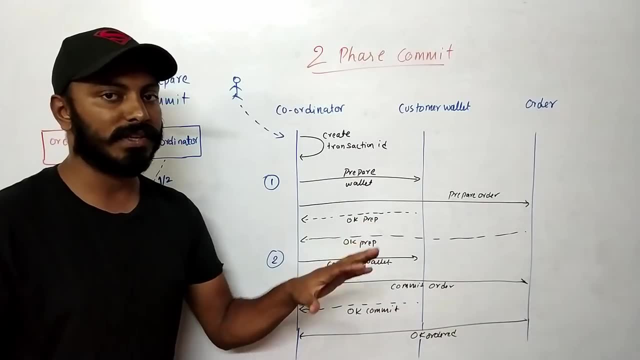 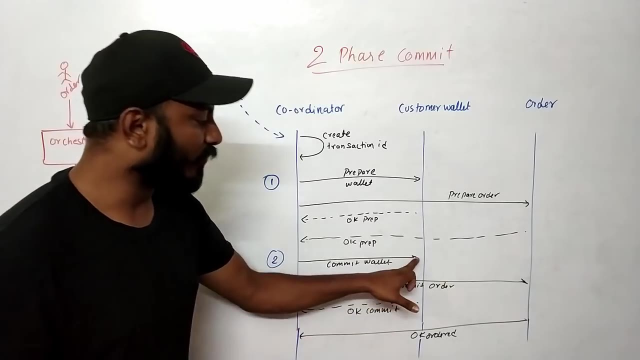 customer wallet and also the order microservices to start coming. what that means? it basically giving permission that, yeah, you guys can go ahead and commit whatever you guys have prepared or locked. then the two calls will be basically placed. one is commit wallet and then commit order. both will basically commit it at this point at the time and then they both have to respond it back to. 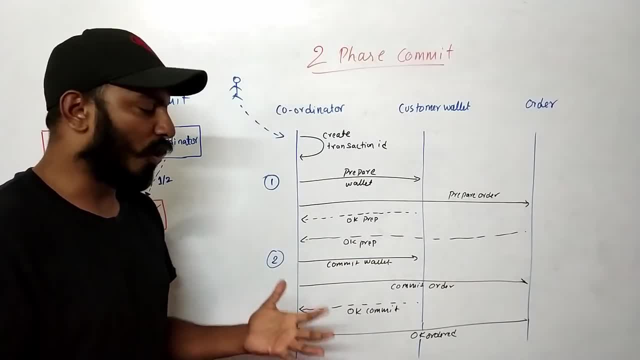 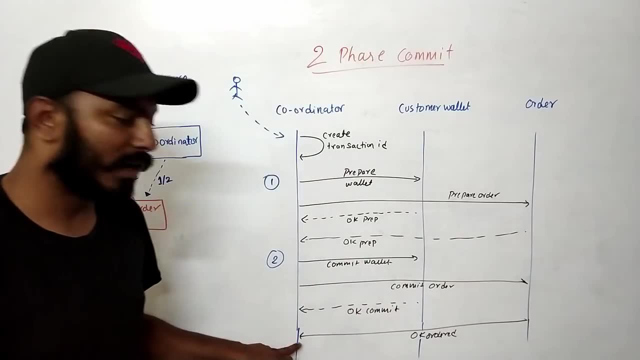 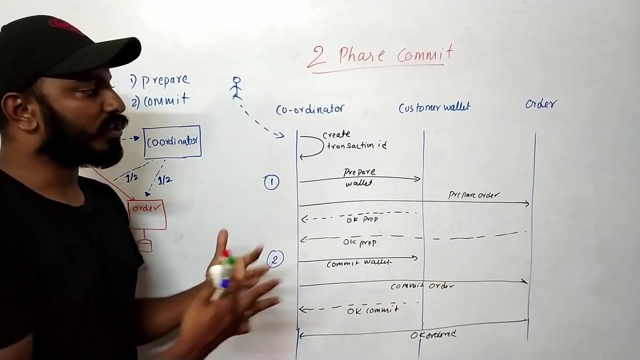 the coordinator saying that: did we successfully committed or not? so in this case, both uh sent back the reply that yeah, okay, commit. and also this guy replied back to the coordinator that okay, we order of the distributed transaction using two-phase. coming Now we'll have to look into the failure scenarios. 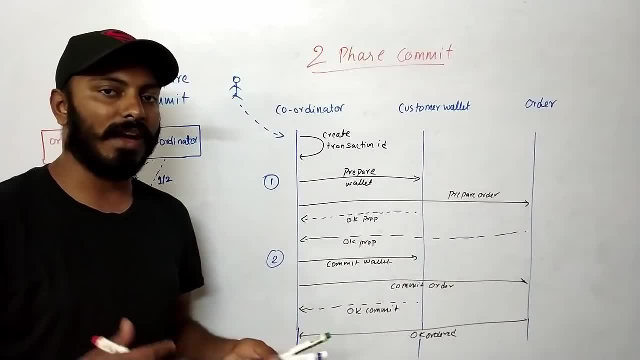 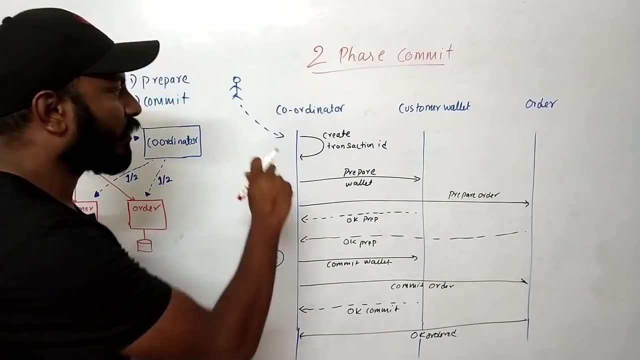 So the first case will be, for example, what if the user doesn't have sufficient balance? In that case, the customer wallet should basically throw an error. So what happens is the coordinator, when he makes a call, prepare wallet. basically this one. 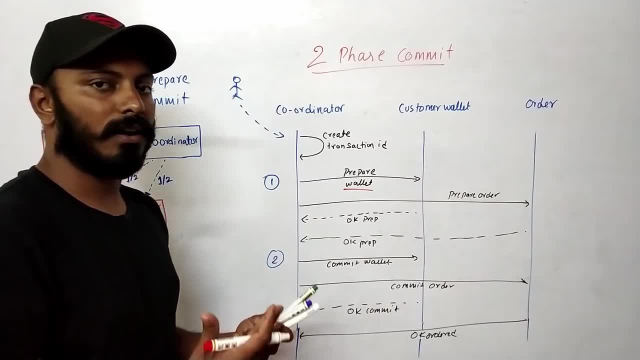 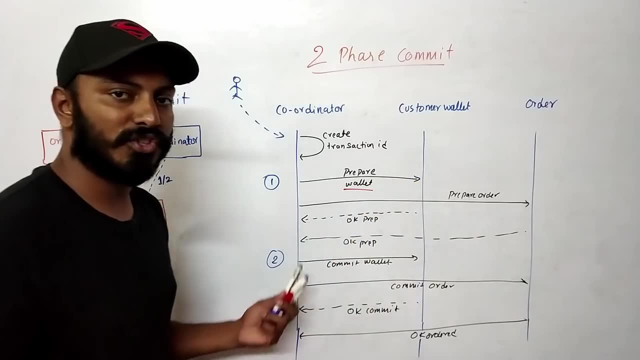 the customer wallet. microservices basically try to check whether the customer has enough balance in his wallet. If he doesn't have, basically in this phase itself he starts to throw an error. How Basically he basically responds: but it's not an okay preparation, okay prepare. 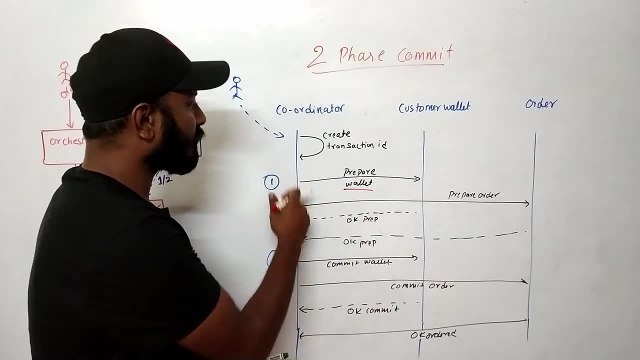 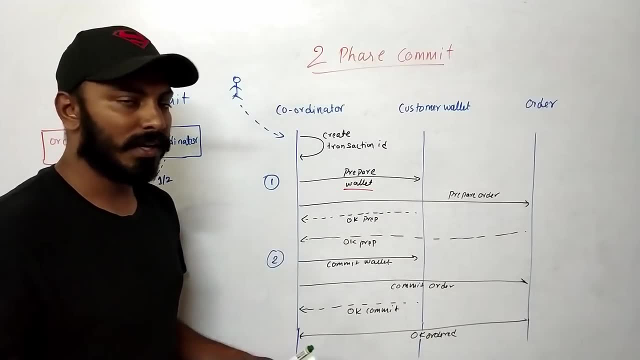 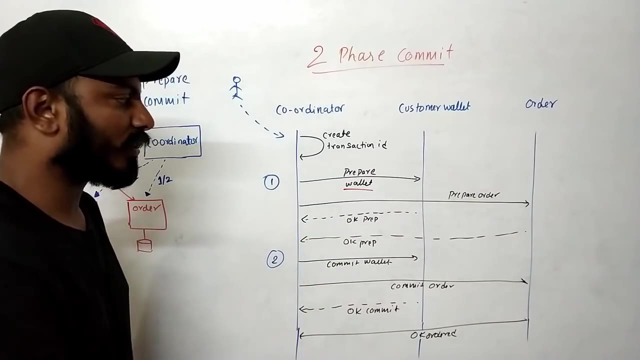 but instead it will be throwing an error And as soon as the coordinator sees an error from the customer wallet microservices, the whole process will be aborted, And that's how the distributed transactions basically handle the failure. In case of preparation, the customer will have a sufficient balance. 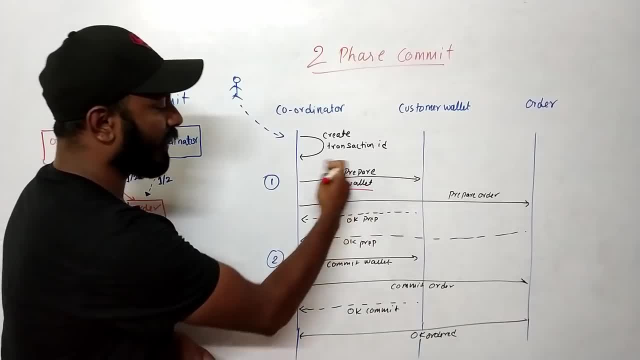 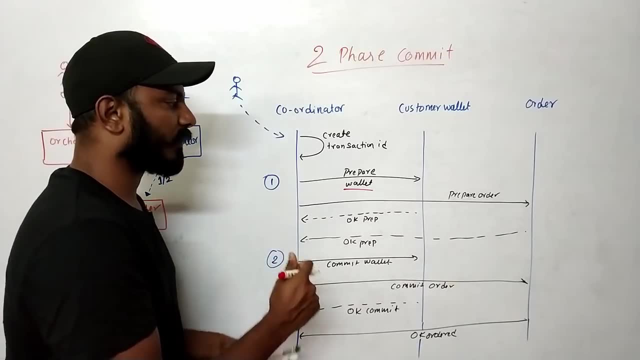 And in the inventory we had the order and the order is not there in the inventory. Basically, in the first step itself, the transaction will be aborted For some reason after prepare statement. if there are any errors, then also there are possibilities. 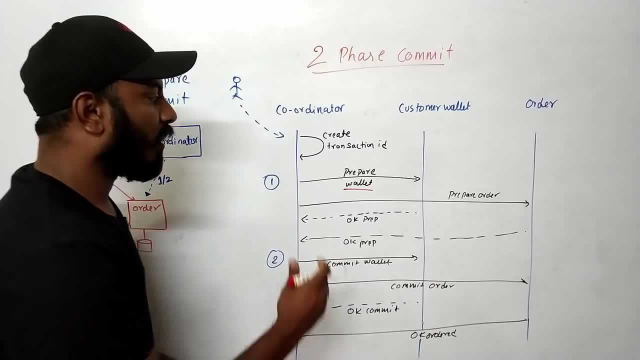 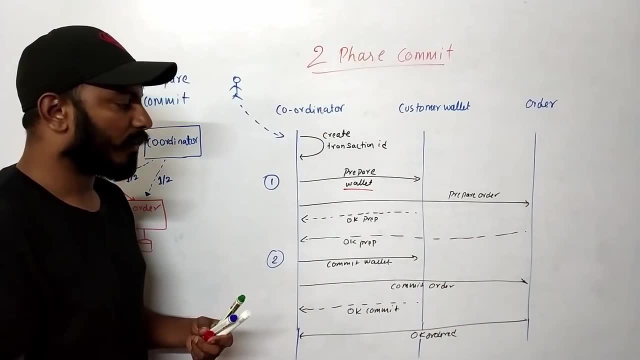 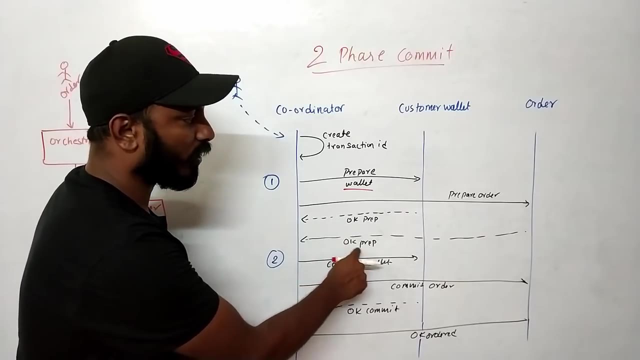 that the whole transaction process might abort, Say in case the customer had the sufficient balance and in the inventory we had the order. so in that case the prepare phase will succeed with okay preparation and okay preparation by the order. So now basically the coordinator. 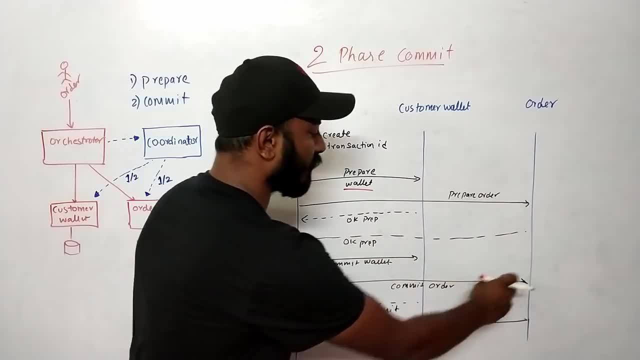 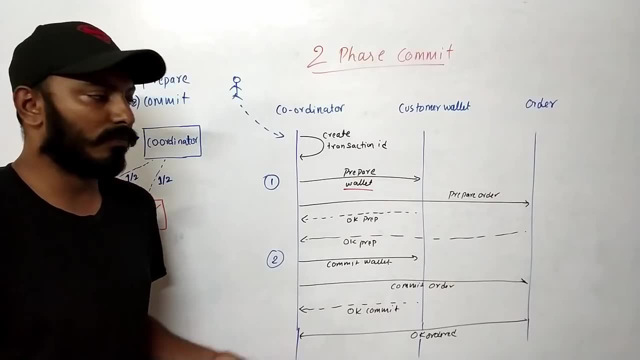 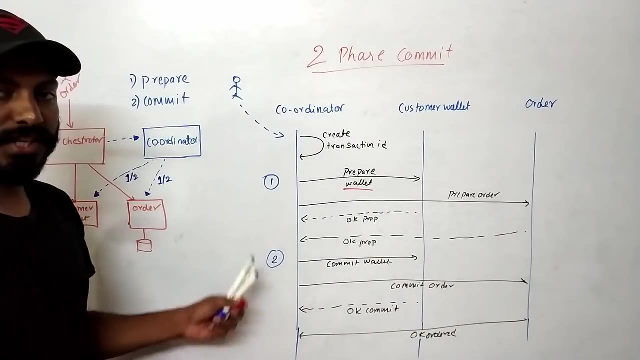 tells customer wallet service and order services to commit it When both guys try to commit. if there is some inconsistent value for some reason, just for example, then definitely the error will be thrown at this stage And again the transactions will get aborted. 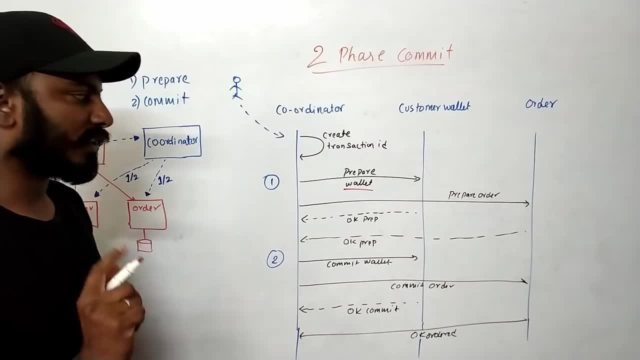 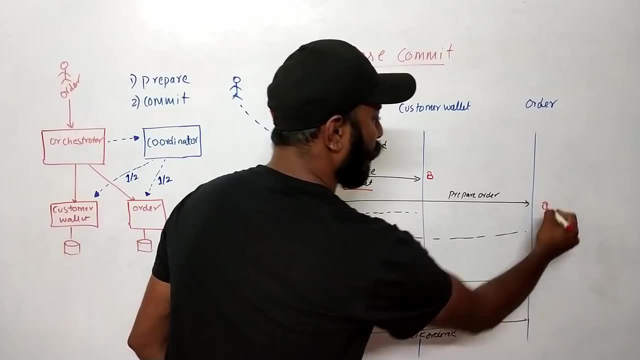 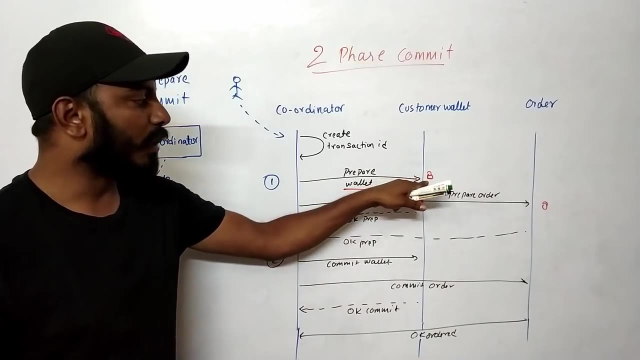 So how exactly the isolation is provided here? Because, as I mentioned in the prepare stage itself, basically both will lock their respective rows using their local transactions, So no other request will basically can modify the same row which is locked. So in case of here, 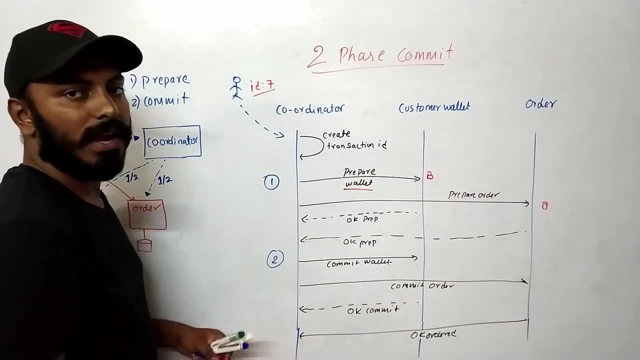 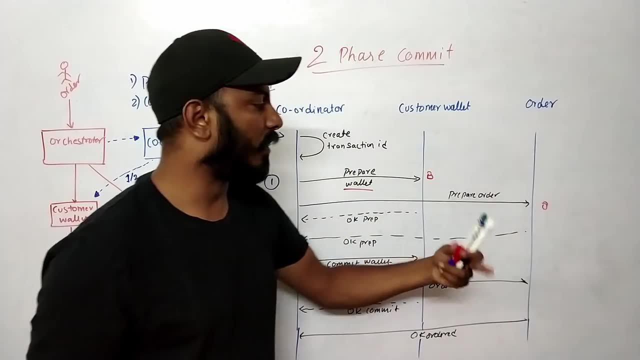 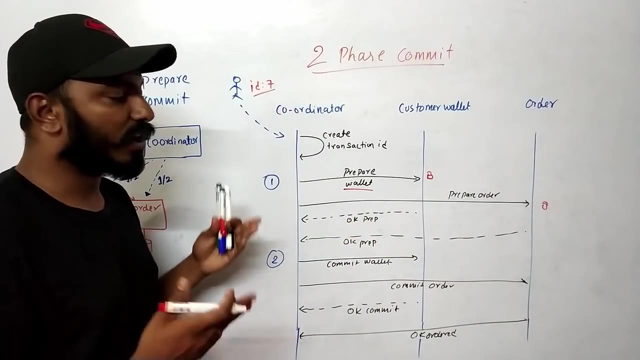 if you are modifying ID 7, so in that case, in the prepare stage itself, the customer wallet for ID 7 is completely locked And the order for ID 7 is also locked. So no other concurrent request will not modify the wallet. 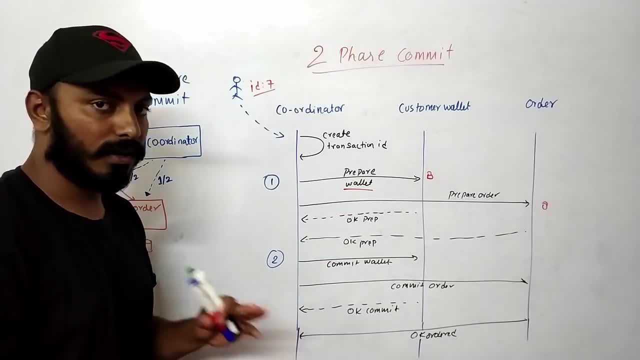 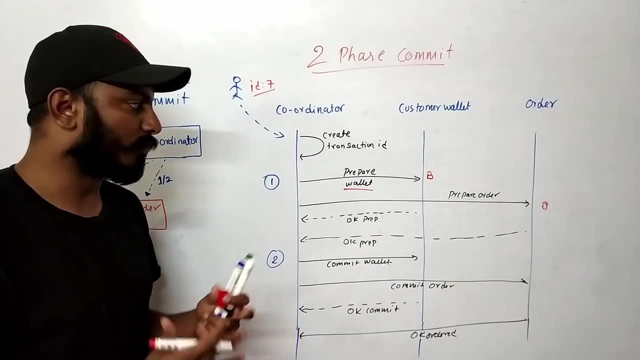 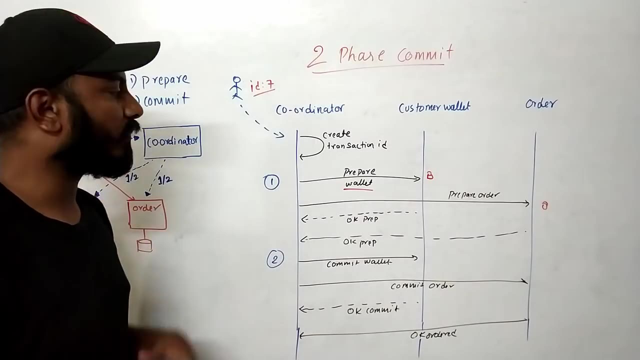 They have to wait until this transaction returns the lock. So that's how the isolation is also provided And the whole thing is kind of behaving as a proper transactions in distributed environment. So the only important thing we need to remember is we need to definitely have a timeout because, say, 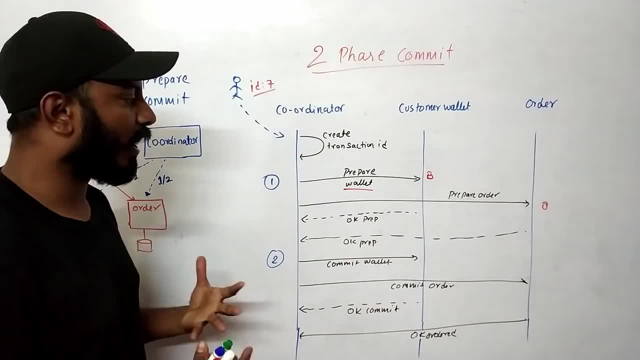 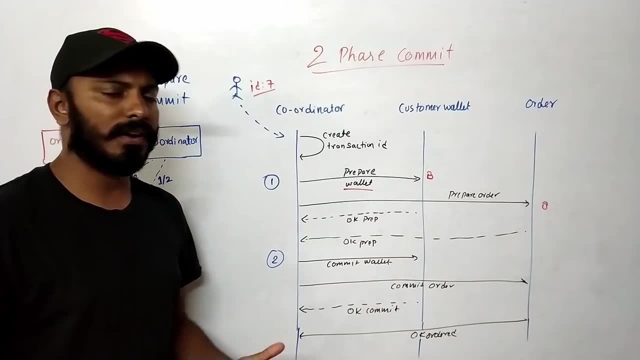 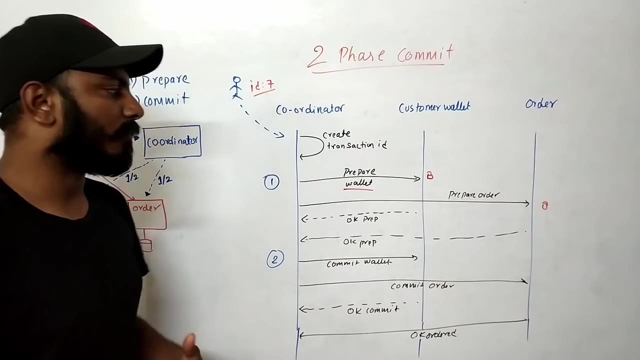 for example, the coordinator should definitely have a timeout. Why? Because he sent a message: prepare wallet, prepare wallet. to both of the services. What if these guys never returned? OK, prepare message. Then it doesn't mean that coordinator should keep on waiting, So he has to abort the whole transaction. 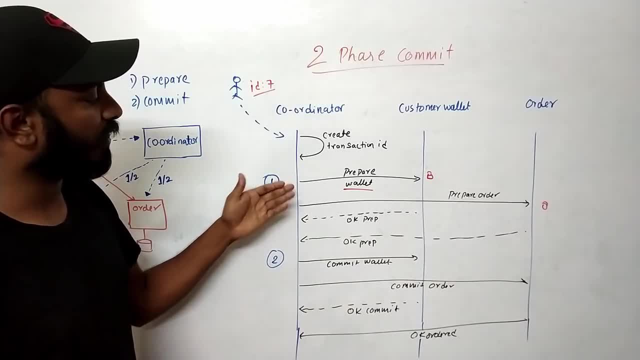 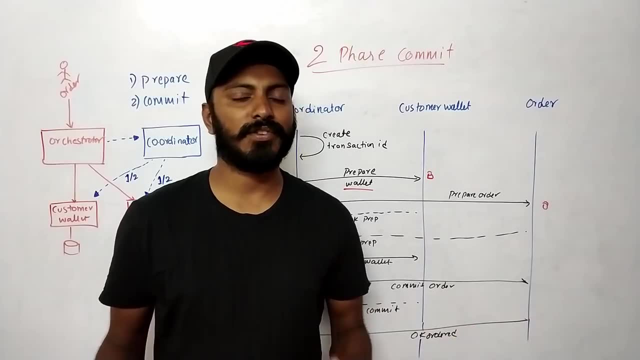 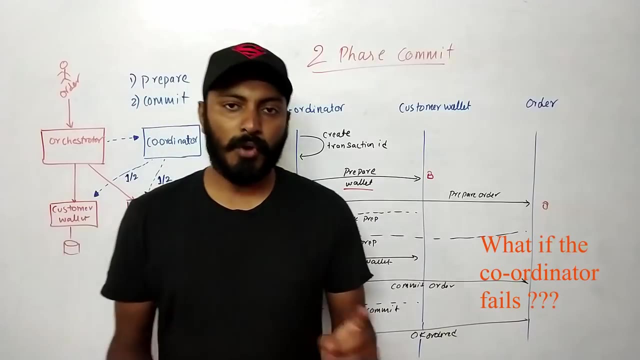 So we also need to set some timeout values for you know, basically waiting timeout to make this thing work properly. What are the advantages and disadvantages? So the advantage is it is definitely a strong, consistent model of distributed transaction. OK. but the problem here is, if you see, it is the 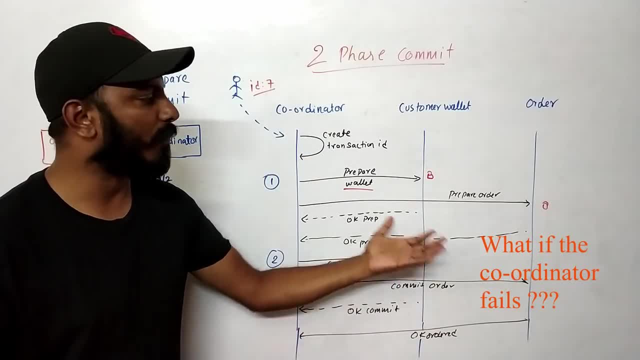 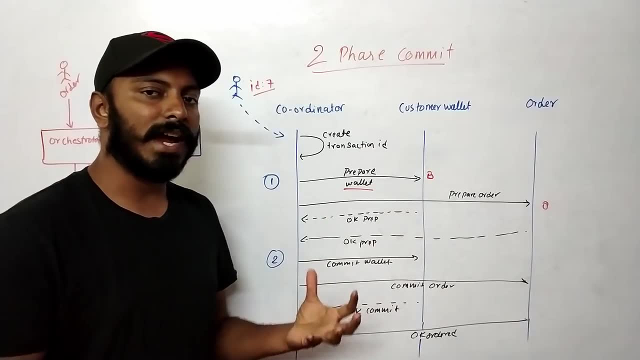 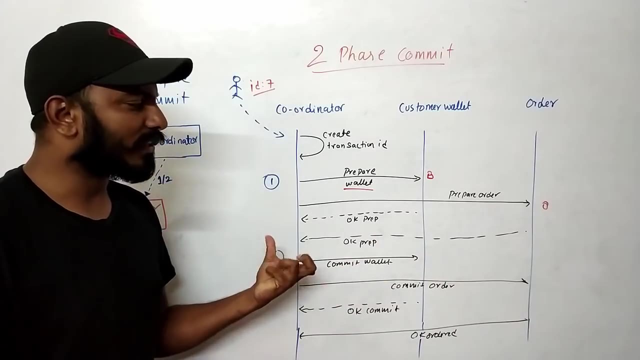 coordinator who is basically handling all of these microservices, and that's kind of bad. And also, if you see in the from the prepare statement, the resource is kind of held up or locked. since all of these dialogues are the talking is happening over HTTP. that that's kind of slow as 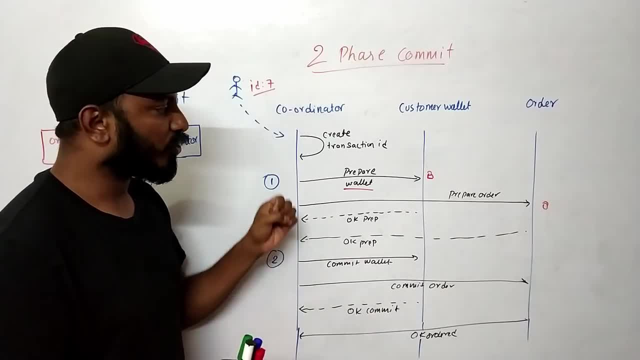 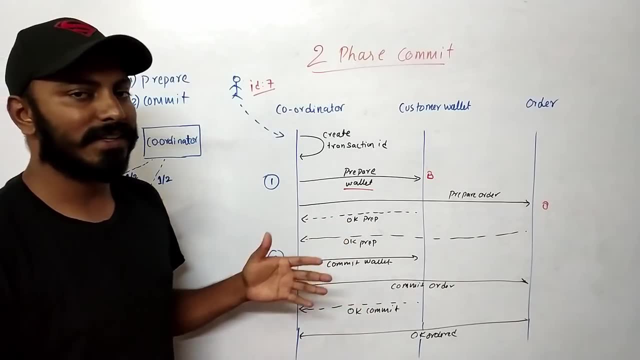 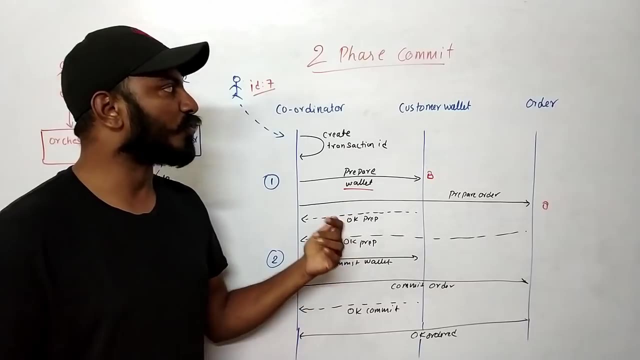 compared to the other database transaction. So these locks are kind of held up for so long time that it kind of causes a lot of latency in the system. And that is the one important reason why people doesn't suggest to use two phase commit in case of microservices. 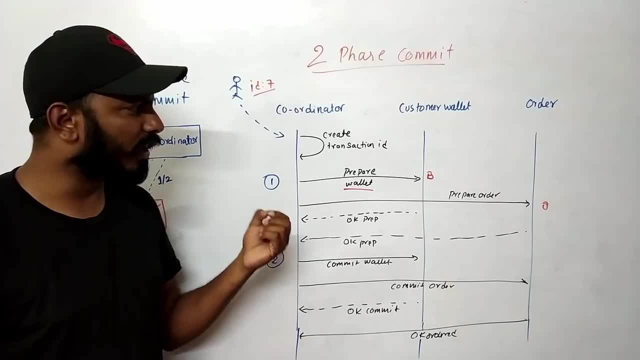 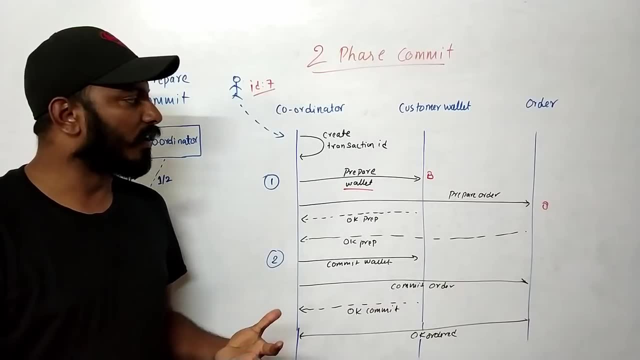 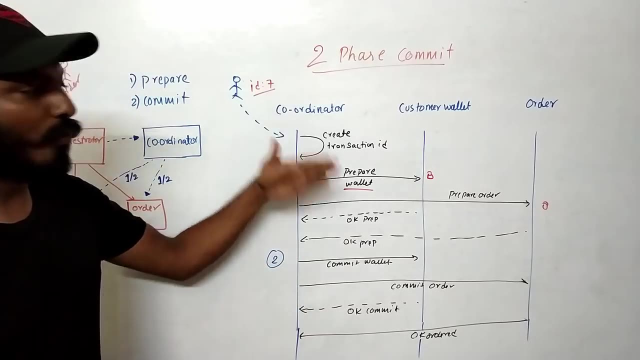 So the two phase commit has strong consistency, but there are some, some serious problems with the way it works And that actually makes the development, developing this particular protocol a little more tedious job. Say, for example, let's go one by one. 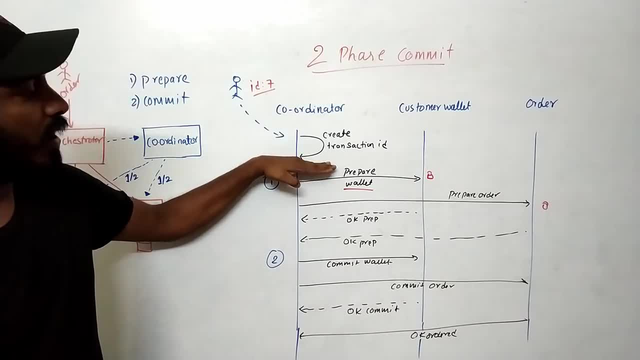 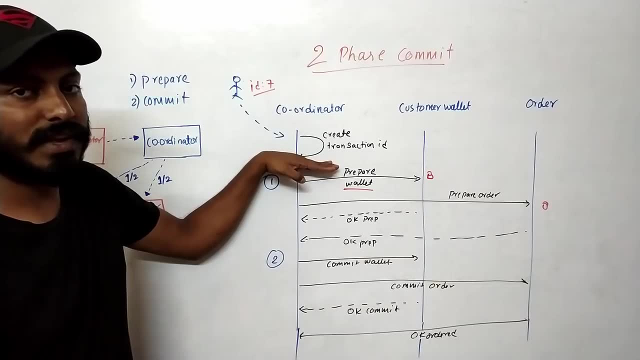 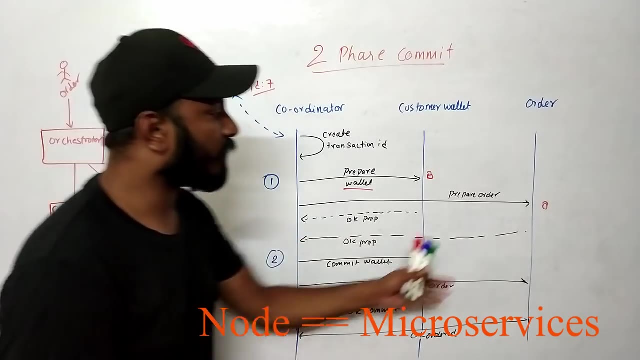 What happens if the coordinator fails? at this stage, We have just created the transaction ID and the coordinator fail. What happens to the whole procedure of distributed transaction? We don't know right. So what happens if, for some reason, the node didn't even respond back when the coordinators sent a prepared? 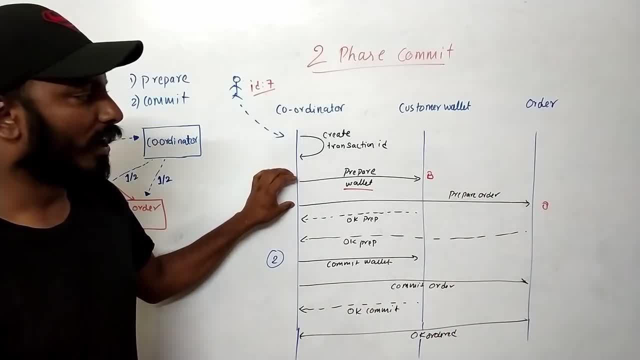 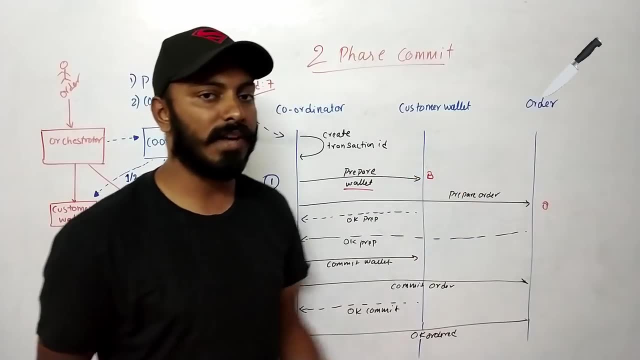 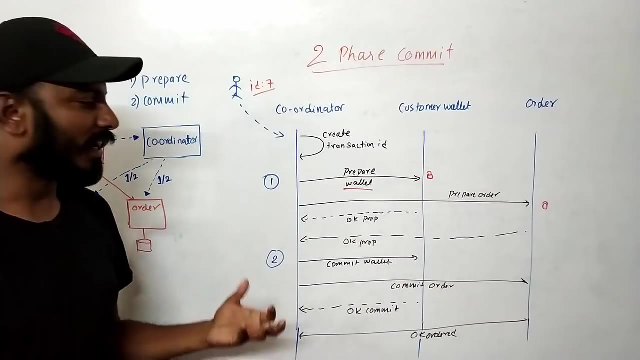 message the coordinator will be keep on waiting, hoping that the order microservices will respond to me. But what if this particular microservices down and he never responds back? So the coordinator neither can't abort or, you know, commit. He has to just keep on waiting. 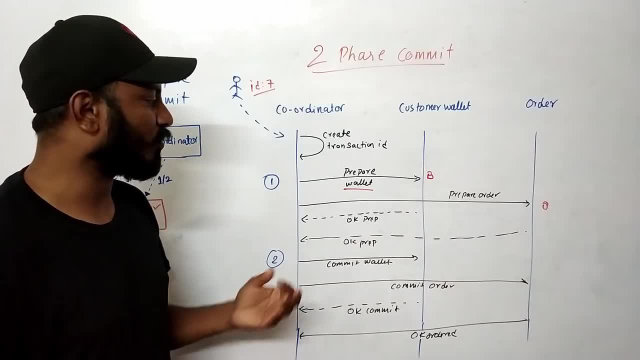 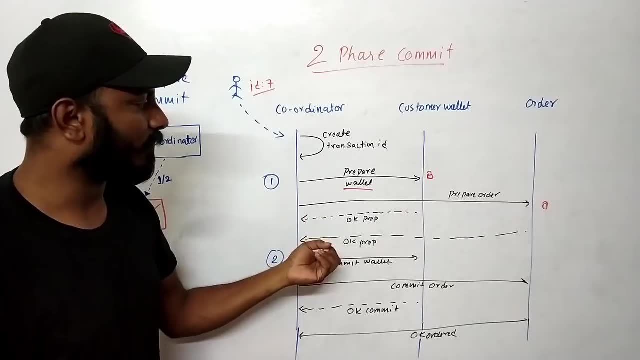 And that is the reason why I mentioned you have to have time out, uh, to not to happen this way, So that some of the other resources will be held um until um, this guy who uh returns an okay proposition message. 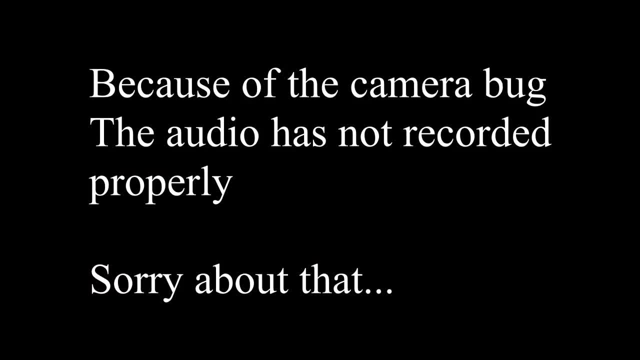 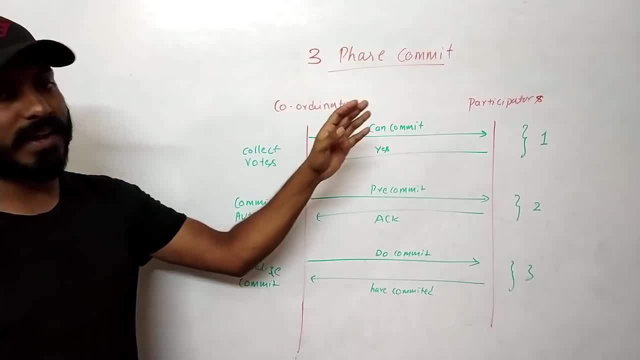 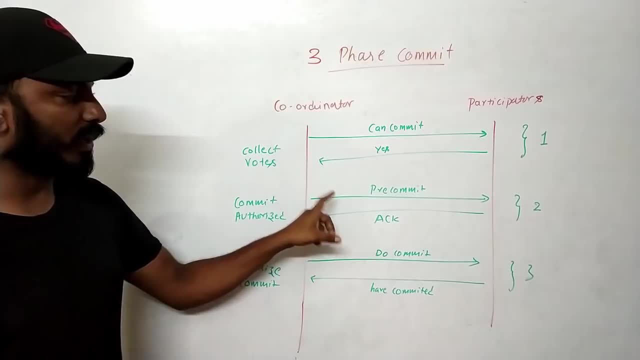 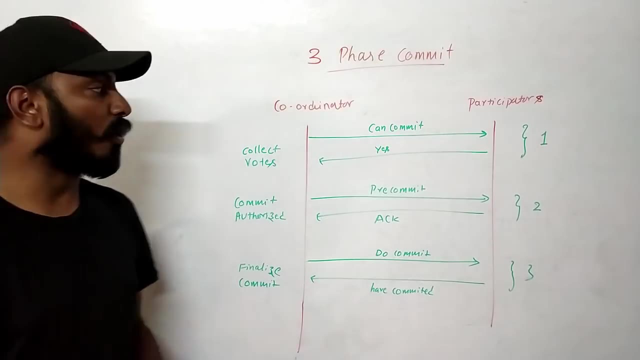 But since this service is- and this is the extension of the two phase commit, called as three phase commit, in which one extra step is included, called as pre-commit step, And having this pre-commit step basically help us to recover in the case of coordinator failure or participant failure. 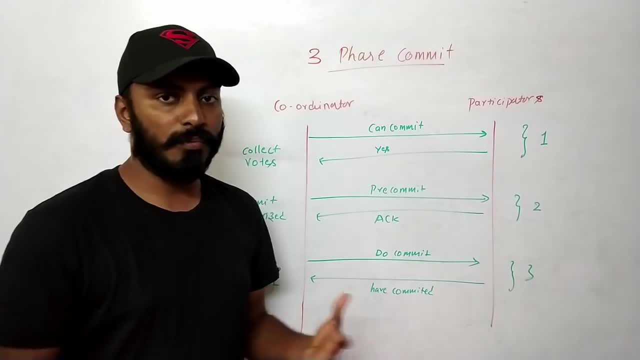 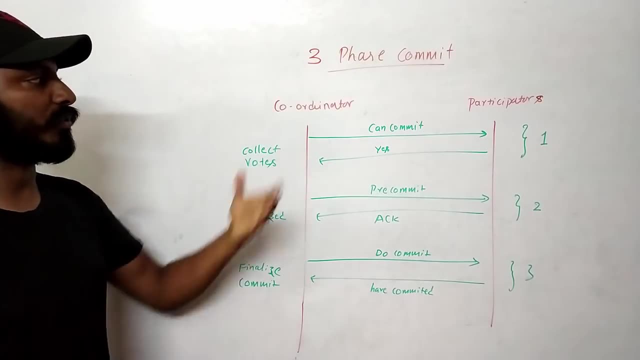 or both. Um, the participators can be one or more. Um, those are the different microservices or different nodes which are actually participating in case of uh for three phase distributed command and the coordinator um in the three phase commit. 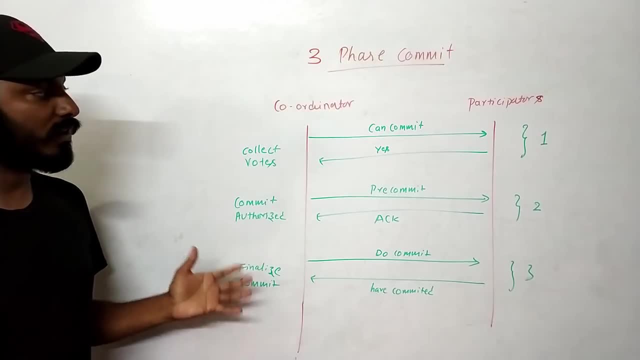 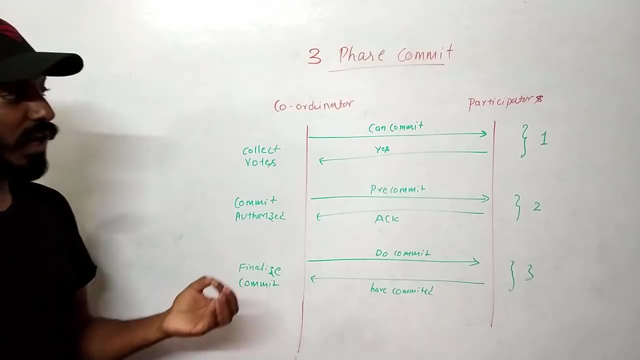 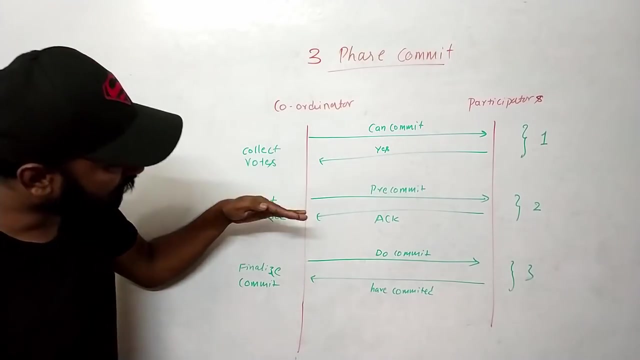 The advantage is: coordinator can be anyone, as I have earlier explained, by leader election, any node or any participator can become a coordinator. And also the advantage is because of the pre-commit, any coordinator, uh, which takes over the failed coordinator, can start from the middle by 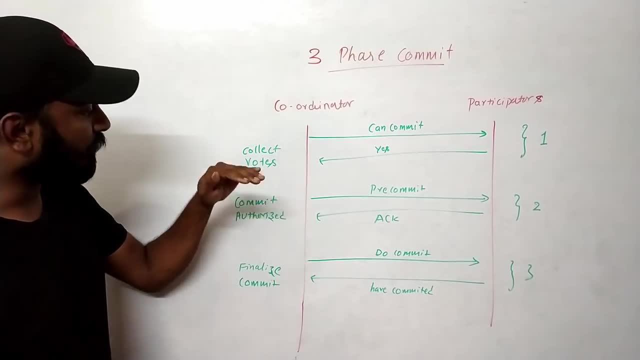 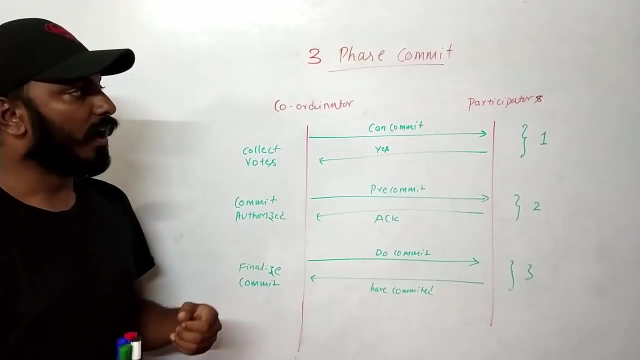 understanding the state of pre-commit. So in three phase. the first stage is called as can commit. in this case the coordinator basically understands how many participants are there And um, so it basically sends a request, called as can commit, and all of the 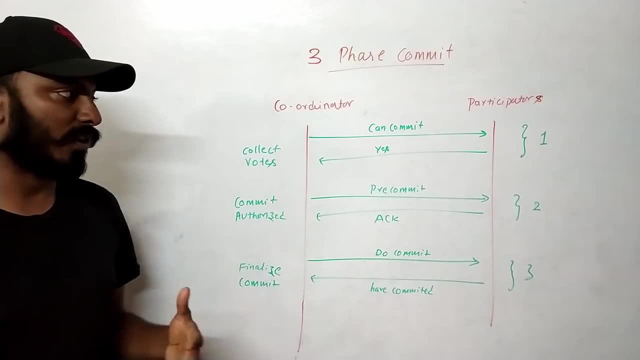 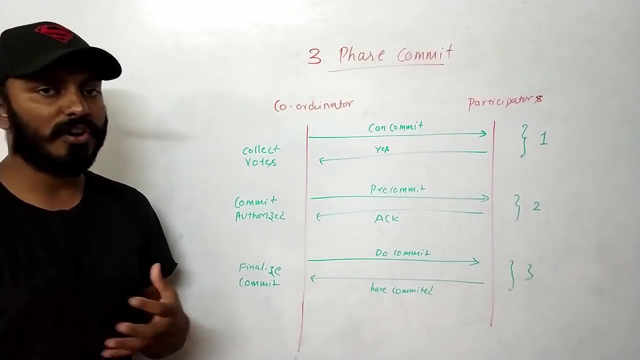 participants reply as S or no or whatever. So that's the first phase, Um, and then in the pre-commit phase, this is where the coordinator basically tells to lock or, you know, to prepare the data to start the commit procedure. 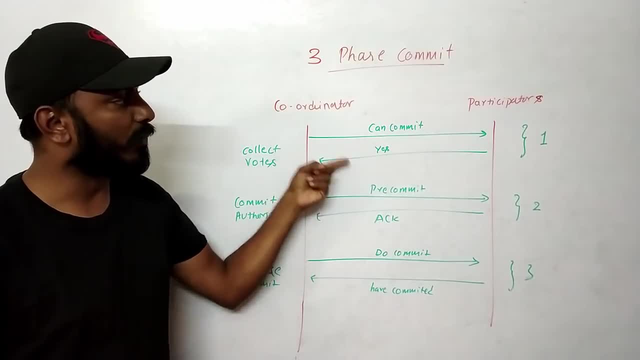 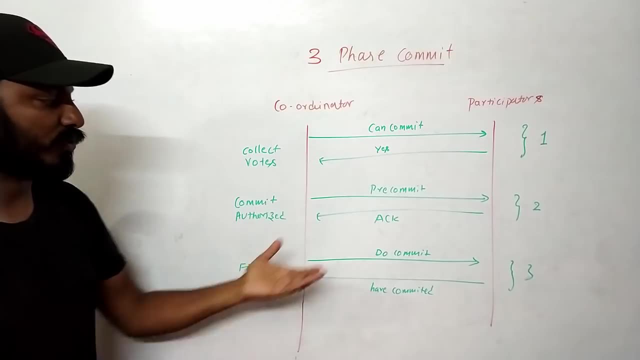 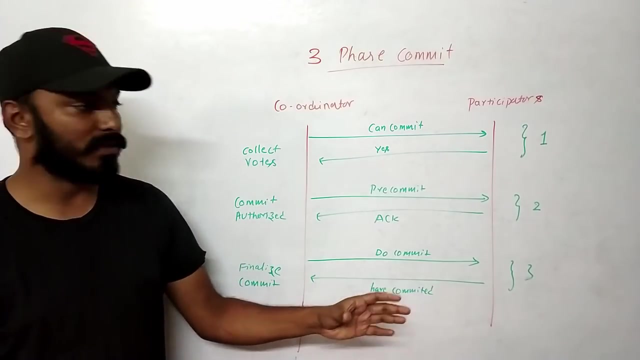 And then, once the acknowledgement is received from all of the participators, which the count we got from the first step. So the coordinator waits for all of the participants to reply to that by acknowledgement And then it basically um calls every participator to do commit and then waits for them to reply. 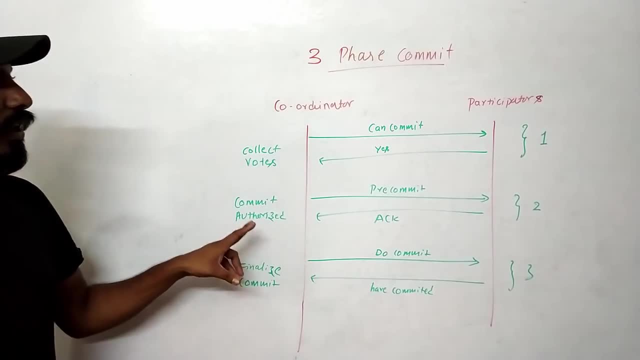 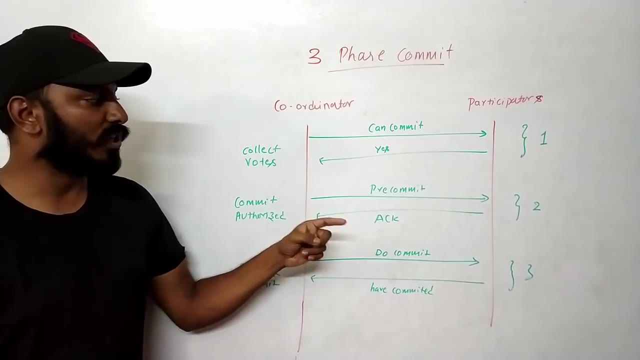 So that's how the three phase commit works. It is somewhat similar to two phase, Uh, it's just that one pre-commit stage is added, And I'm going to show you how exactly this stage helps you to, uh, take over when some 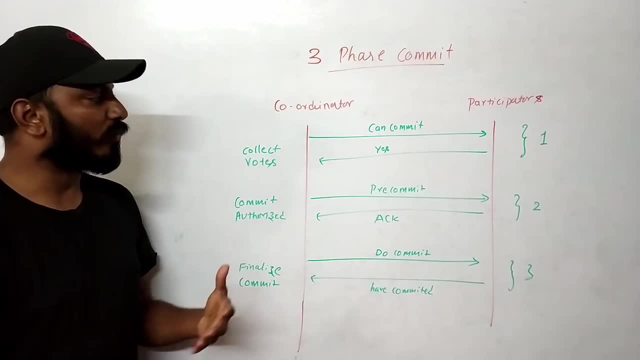 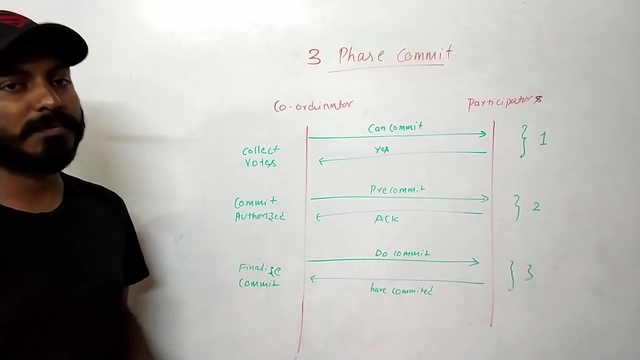 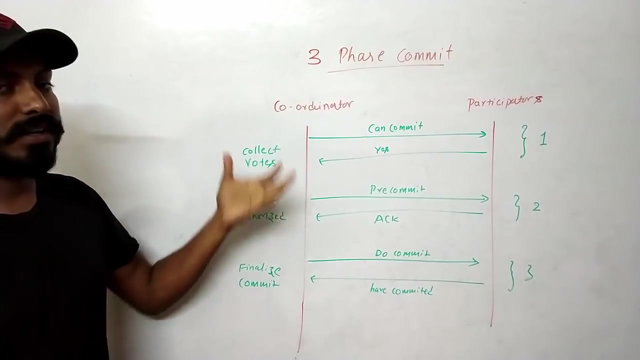 uh, you know, coordinator or participator fails. So let's see how three phase commit helps us to recover from the state where the earlier coordinator died. and, uh, um, how new coordinator will exactly take over. So let's see how three phase commit helps us to recover from the state where the earlier coordinator died. and 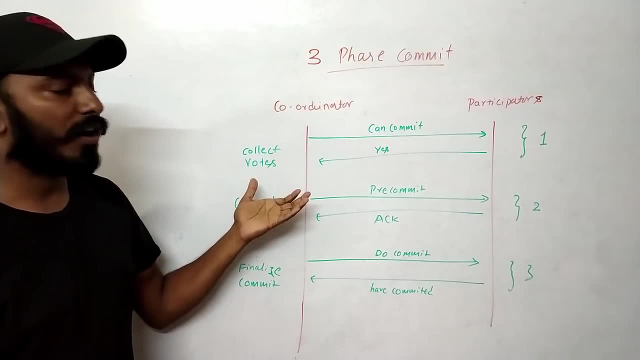 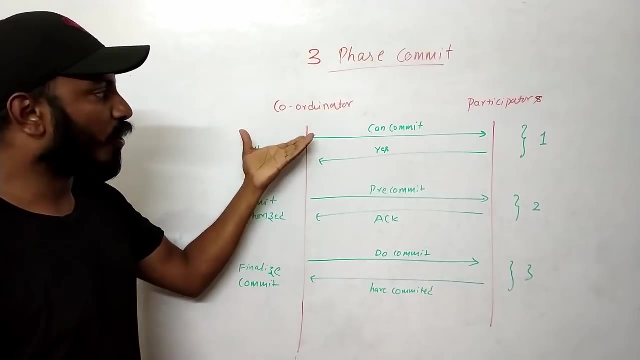 uh actually take over the that state. The new coordinator definitely needs to talk to all of the participators to understand the state. Say, for example, if the coordinator uh, when the coordinator talked to participator, if at least one participator says that I have the do commit. 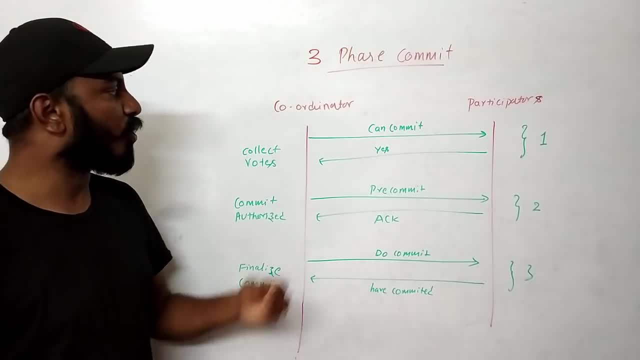 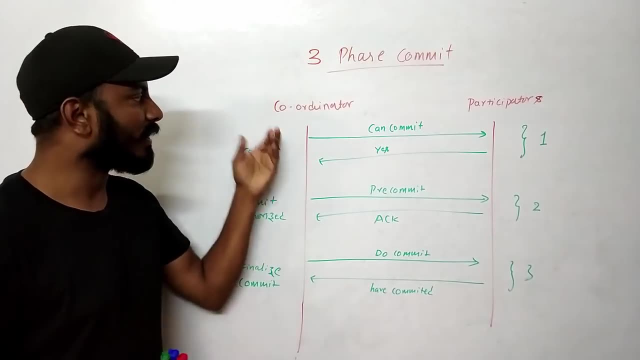 um, you know, message received. that means that for sure the new coordinator can guess that the old coordinator was definitely ready to issue a do commit And hence the coordinator can take over from there by issuing do commit to all of the participants and committed for some reason. 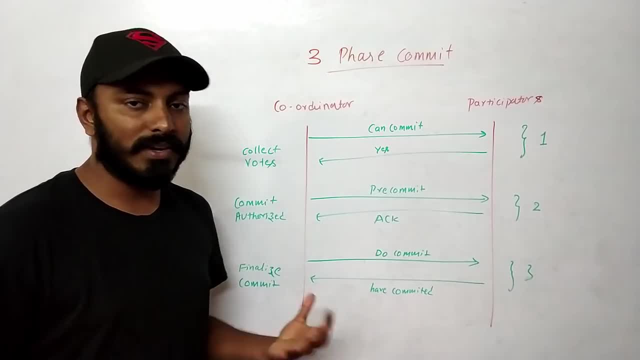 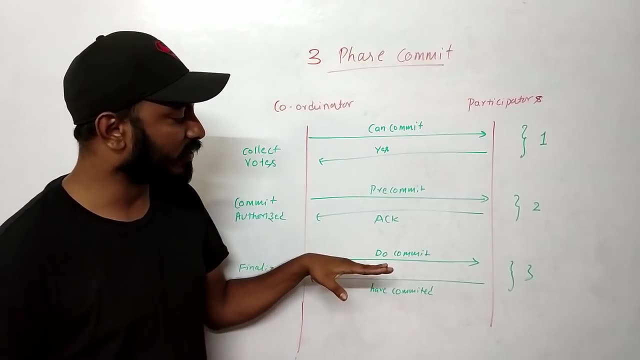 If none of the participants says that I haven't received pre-commit, that means that for sure the new coordinator can guess that none of the participants- uh, participators- would have committed the data. So that means that we can either start from pre-commit stage. 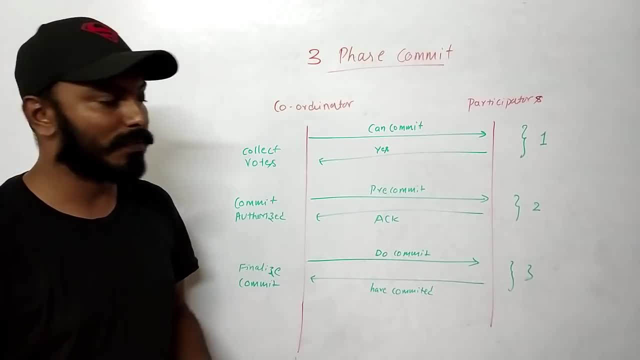 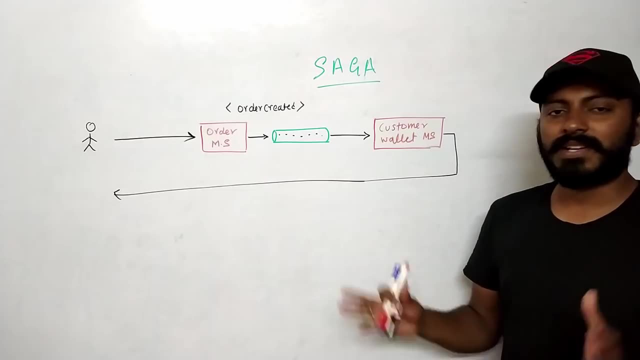 or we can start over from the can commit to understand how many participants are there, And then the pre-commit stage will continue and all of the data will stay consistent. We learned two-phase commit, three-phase commit and also dynamic way of choosing coordinator, and all of that. 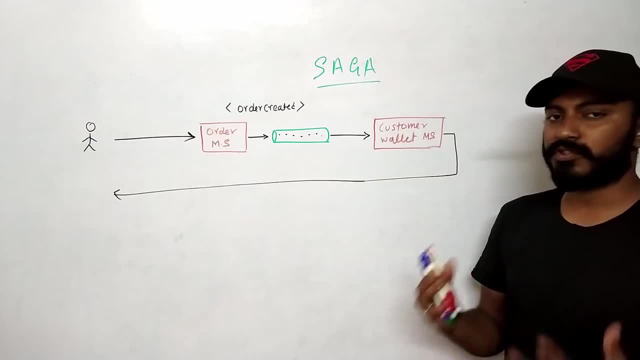 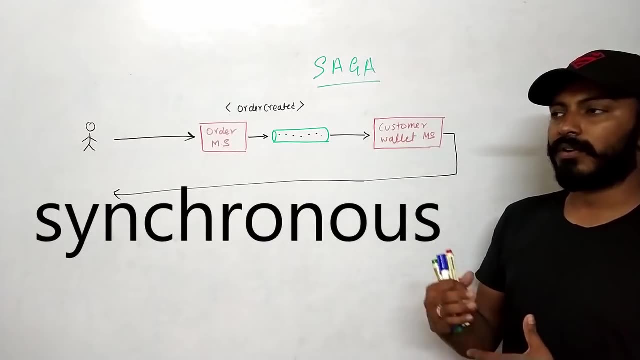 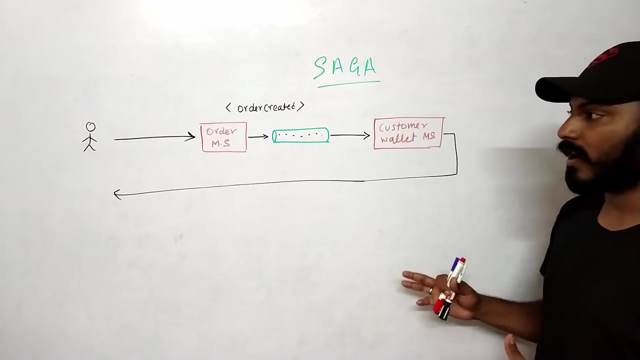 They are good, These procedures works well and they are strong, consistent, but the only drawback is they are synchronous And also they take take a lot of time. That means that increasing the latency. This is also a widely used pattern, called a saga. 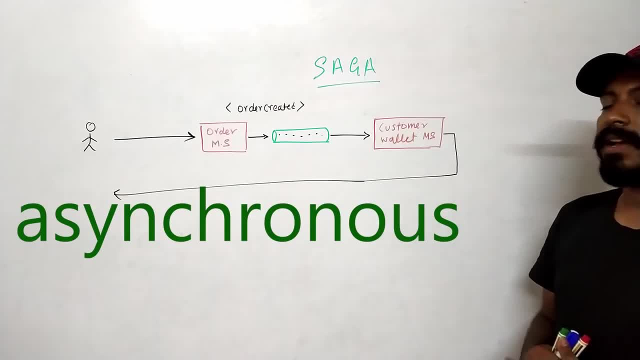 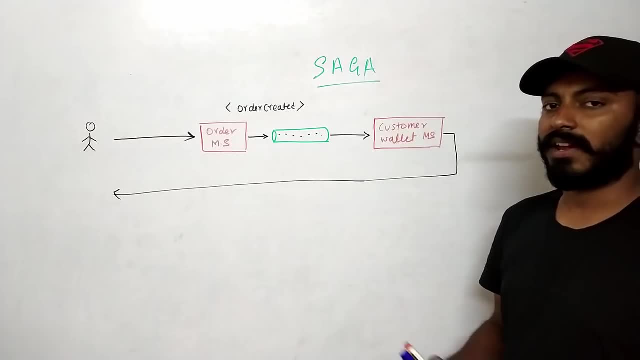 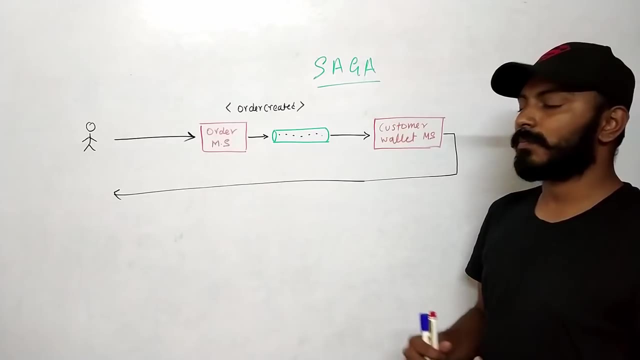 and this works asynchronously. That means that we can implement this kind of pattern when we have web sockets or long polling or even in case of polling as well. it's up to us to choose what kind of technology, but it works well with the asynchronous way of sending the messages between client and the servers. 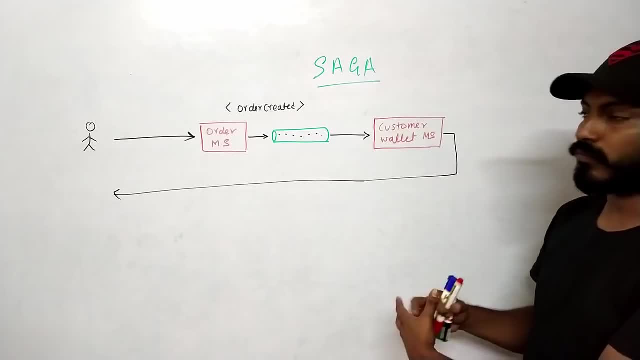 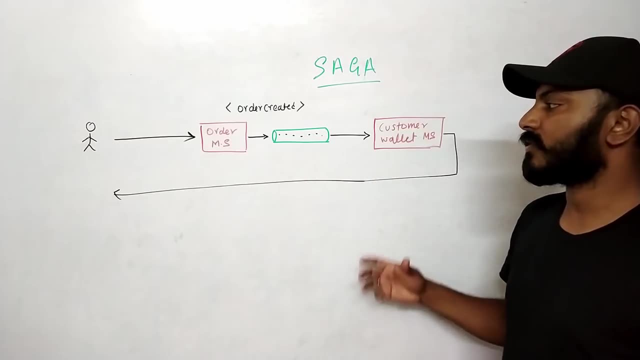 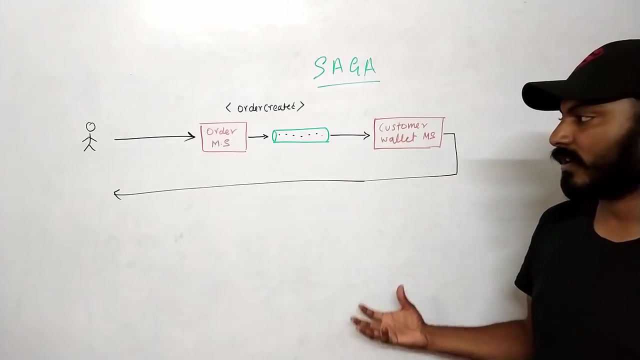 But nevertheless, um the how, how this pattern works, is it the series of microservices basically talks to each other using messages, or even bus or queuing system? Um, let's take a. let's take the same example of placing an order in Amazon or in an e-commerce site. 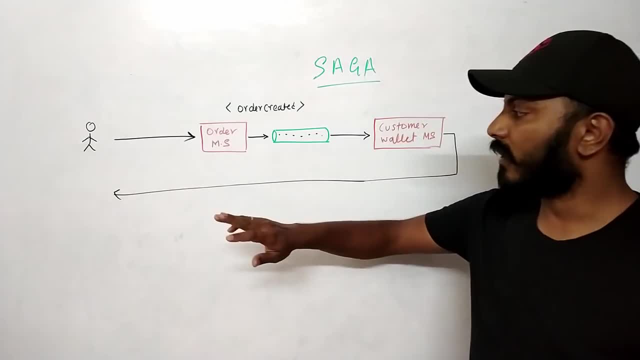 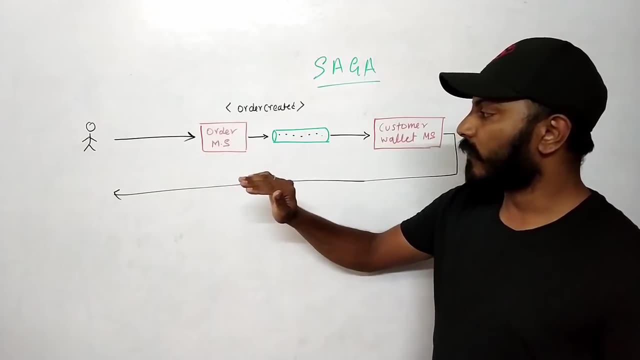 How does it work when the user places an order? Um, the request actually lands up to order and miss, or it could be vice versa. Let's take a. it came to the first microservice, called as order microservice, In this case. 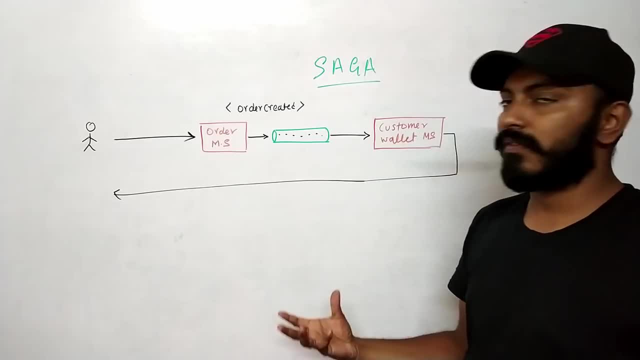 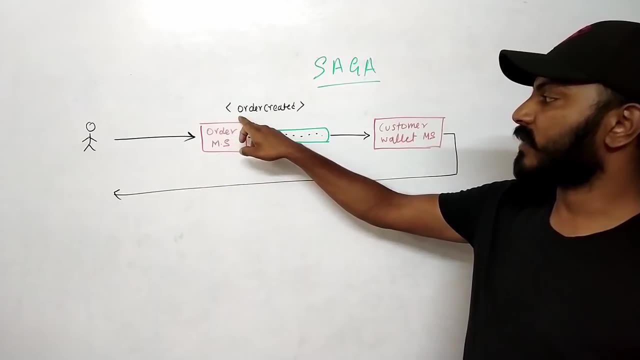 the auto microservice basically checks, uh, the inventory. If it has the product which the user is requesting for, he basically adds a message called as order created into this queue. or it's an even bus, Uh, let's. let's take this as a simple queue. 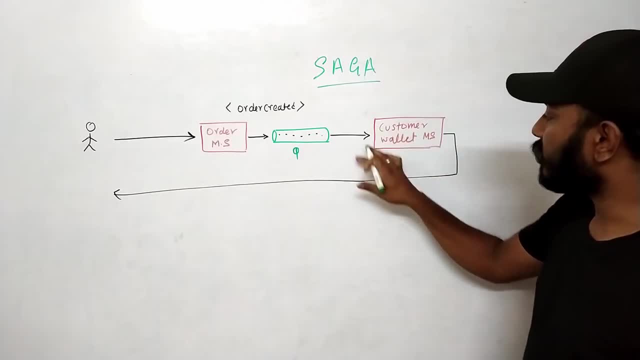 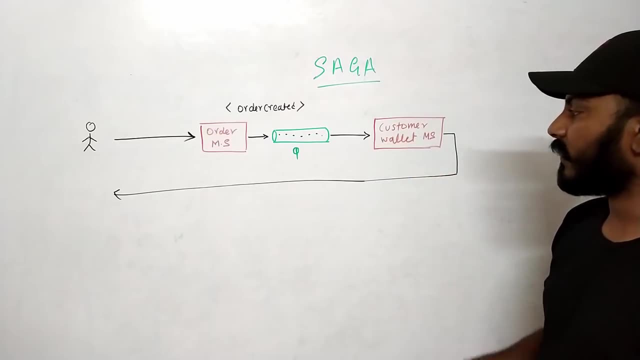 It adds that message over here And then, when the customer wallet microservices is free, it basically picks up message and then processes, uh, by deducting the the respective amount from the wallet. So if all goes well, everything is succeeded. 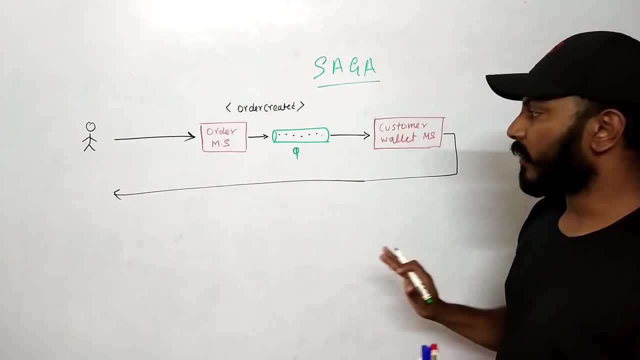 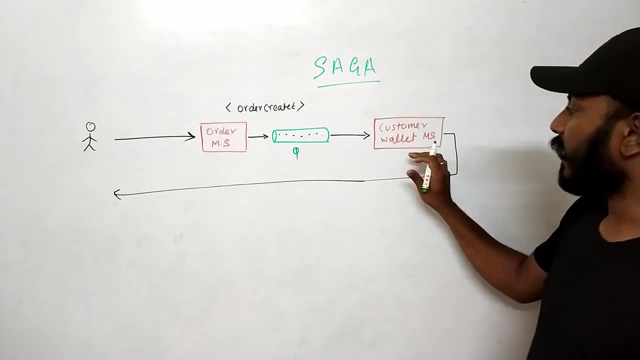 So the whole cycle is kind of finished. What if, for some reason, if the customer doesn't didn't had enough money in his wallet, then this guy will add a message to a different queue. Basically, basically, we need to roll back the order. 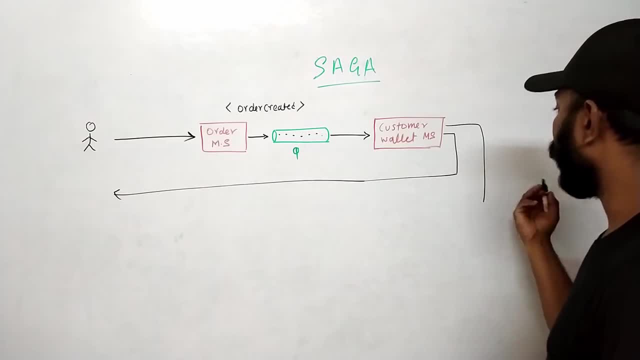 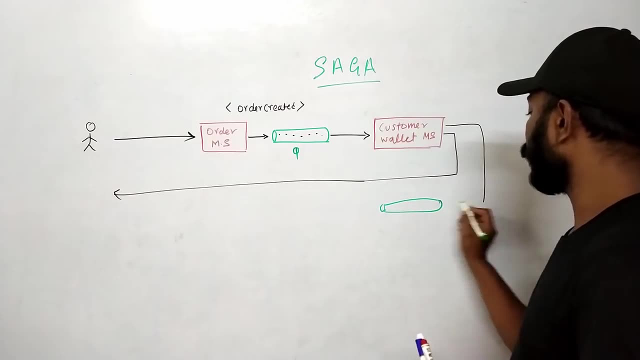 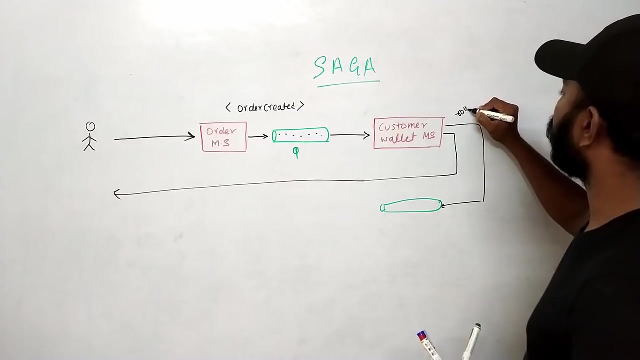 which is space, right, So in that case we'll have one more queue. Um, maybe, maybe somewhere here. So we have one more queue. So so, basically, this customer one, it will. it will add a message called as roll rollback order or something like that. 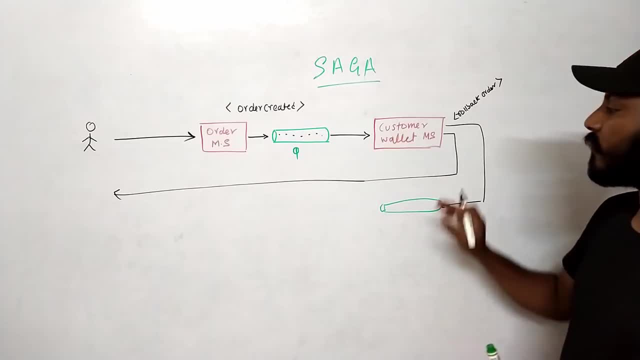 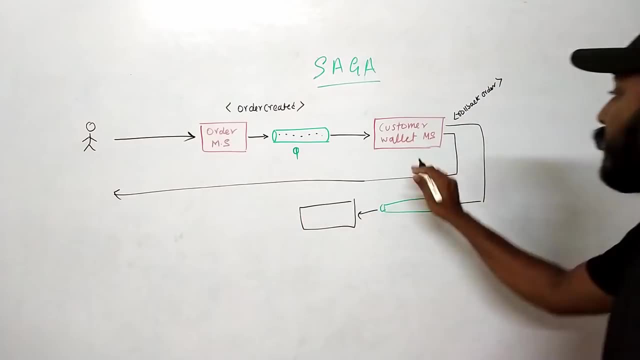 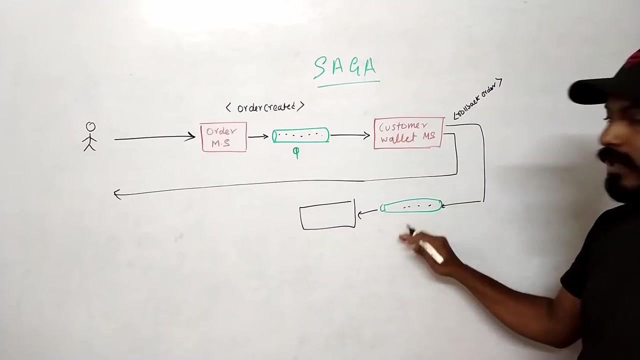 So if, basically for any actions, we need to add a message to the queue and there is a respective microservice which basically takes care of that, So when this customer wallet microservices fails, it adds a message called as rollback order, This message will come and land up into this queue. 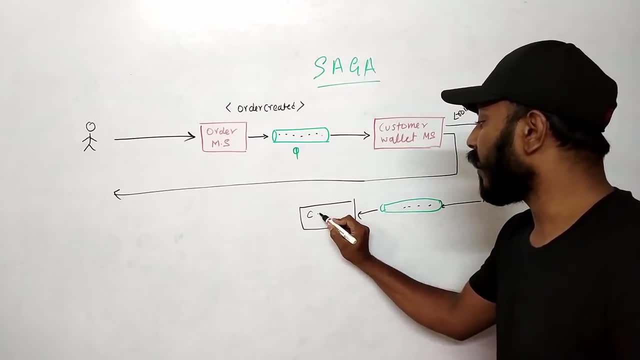 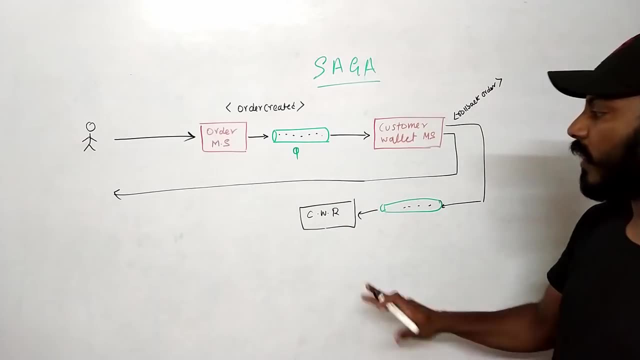 And then there is a microservice which basically takes care of that. So this is basically the order of customer wallet rollback microservices And this one basically does the rollback of order and everything. So they need to be a lot of microservices to take care of. 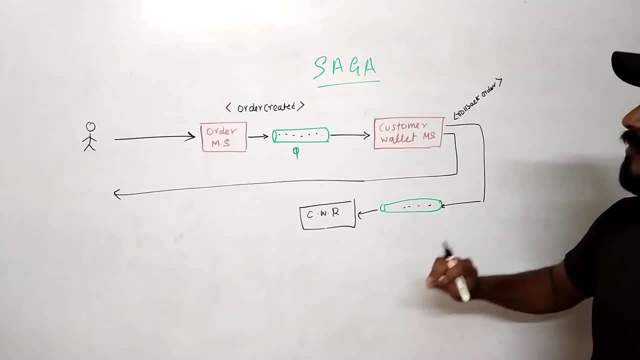 different kinds of actions And all of these actions are basically transferred through the queue or even buses, And hence there is an incident, is a synchronous way and it is little faster compared to the two phase and three phase because we aren't using a lot of. 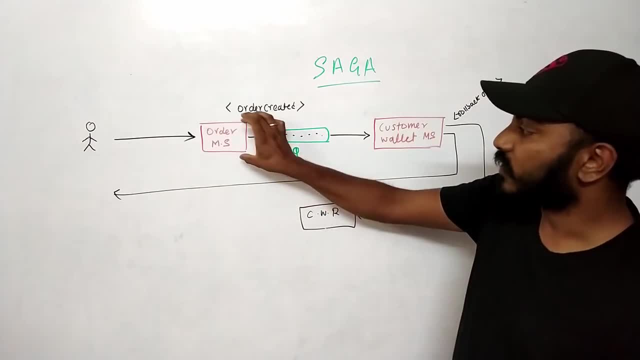 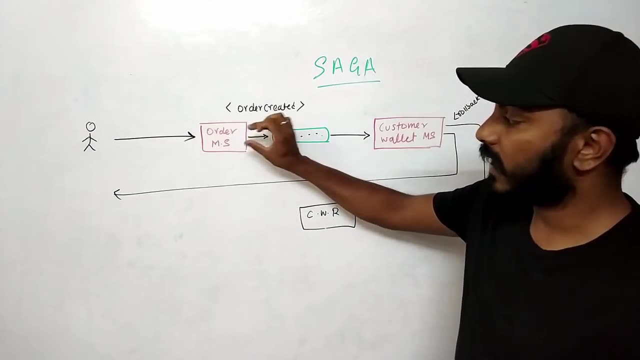 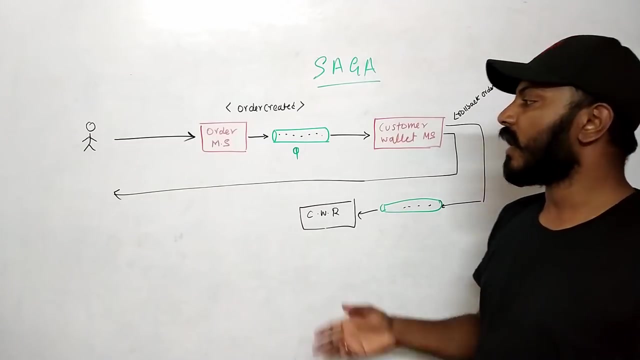 uh, locks over here And all of the transaction is local transaction with respect to those microservices. So when it plays the order there'll be a transaction inside this microservices, not the transaction on all of the microservices, And like the two phase and three phase. 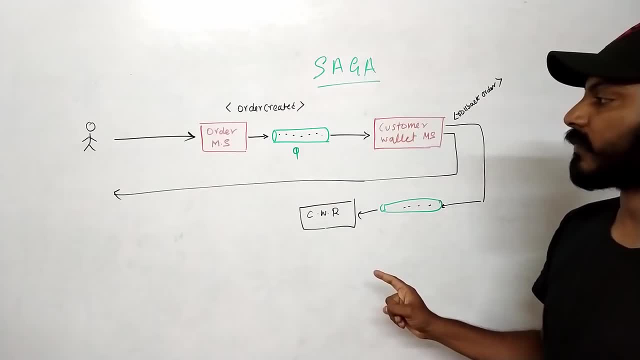 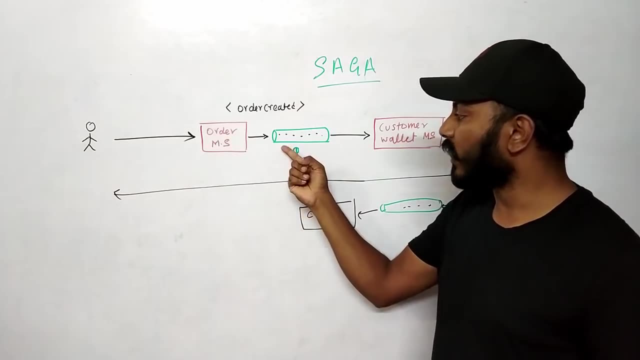 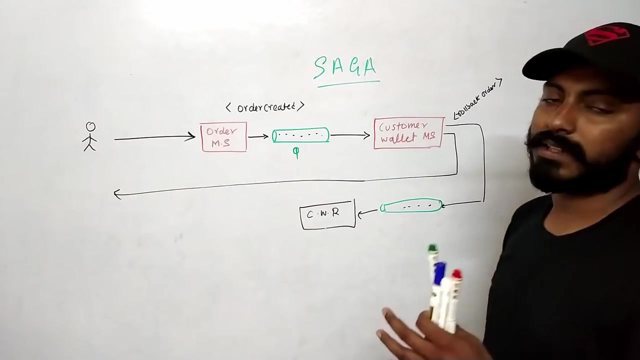 that's why it is much faster and asynchronous, And also how isolation is provided. since any order um requests are going through the event buses, all of the messages are sequential in here And that's the reason why the microservices will not get the 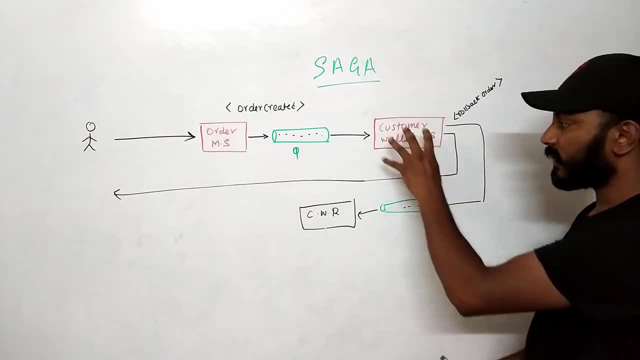 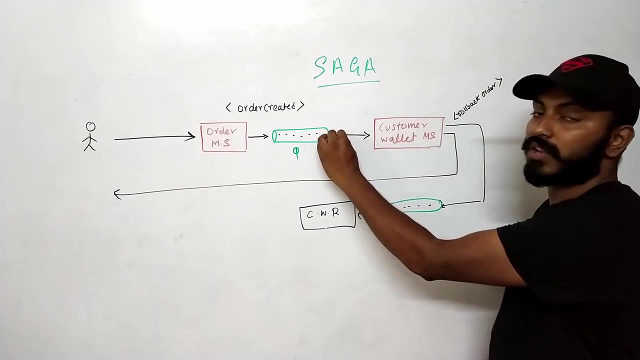 uh, multiple requests at a given point of time. You can scale these microservices into horizontal, horizontally, And uh, these microservices basically receive the sequential messages and hence there'll not be a, you know, isolation problem, um at all. 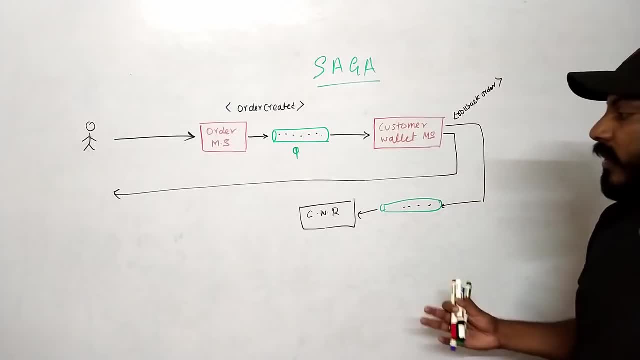 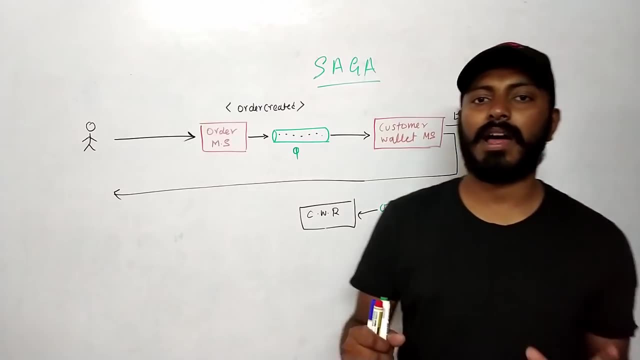 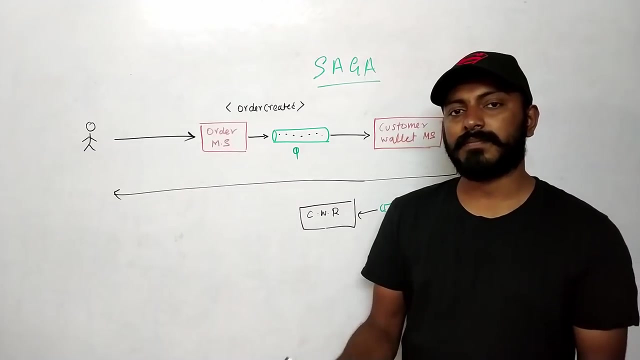 So the complete atomicity will be still provided using this way. So, um, I think that's it. Um, this kind of pattern works well as well. I think uh have covered uh different ways of uh handling transaction in distributed systems.